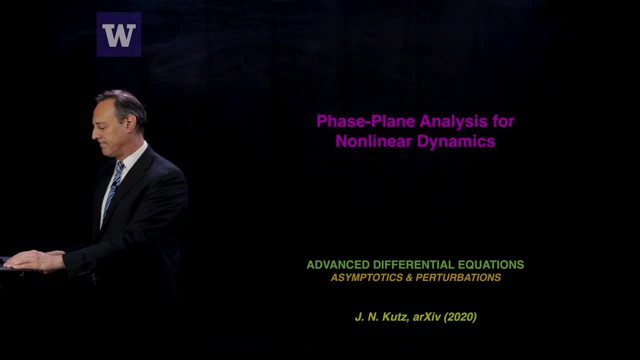 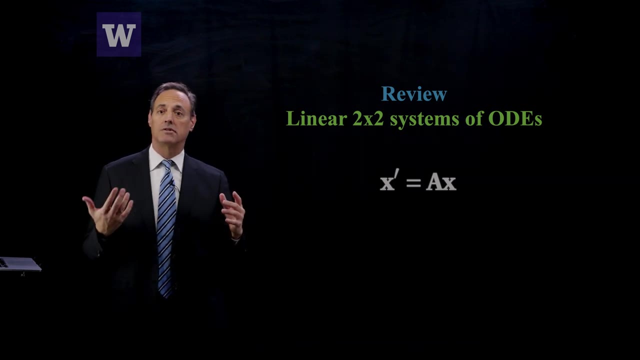 the archive for this course. So let's start off with a simple review of two by two differential equations that are linear and constant coefficient. So the easiest way to write that down is: x prime equals ax, where a is a two by two matrix, And there's only certain things that can. 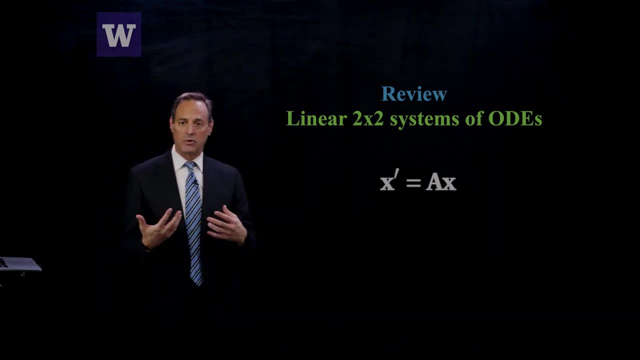 happen in such a simple system. So it's two by two and in fact we have analytic solution techniques available to us which can be found typically towards the back of most differential equations books, thinking about systems of first order differential equations. In fact, second order differential equations can. 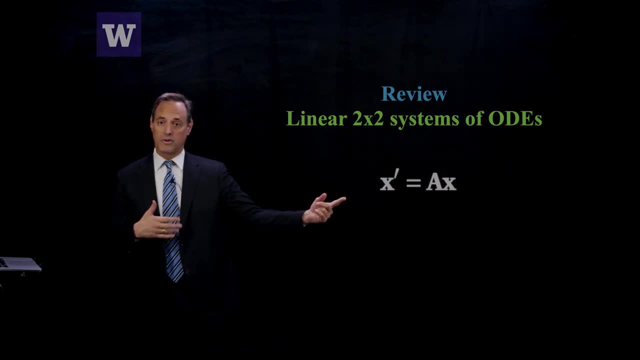 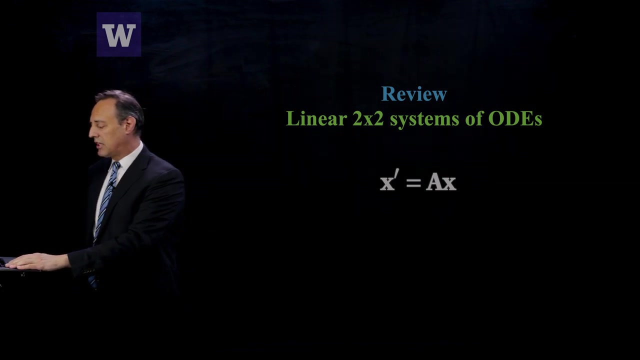 always be written as a system of two by two, First order differential equations, And so this is the generic representation of what we want to consider in terms of looking at dynamics and the idea of a face plane. So we're going to introduce some concepts. In particular, we're going 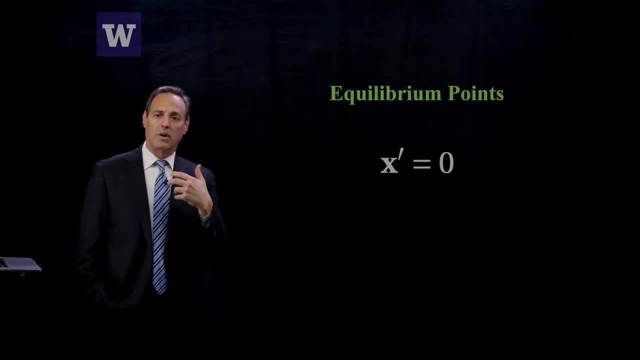 to look at this thing and start thinking about one of the important classes of solutions, or what are called the equilibrium points. We look at: when does x prime equal to zero? In other words, when x prime is equal to zero, nothing's happening, Nothing's changing in time. So this is very much like when. 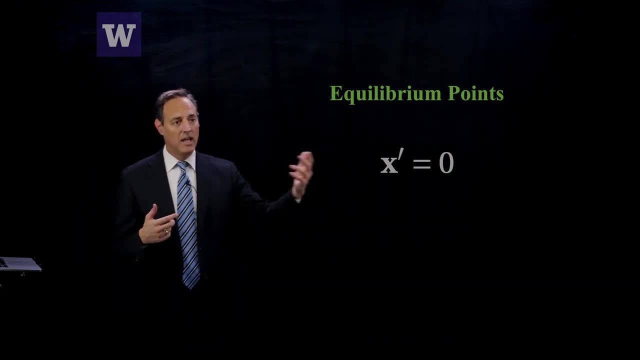 you look for derivatives being equal to zero, which are min and max. X prime equals zero are often called the equilibrium points, In other words, where the dynamics is not changing. So x prime equals to zero is where this happens and there's 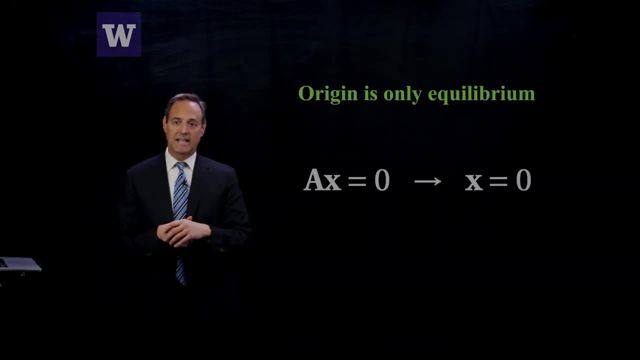 only one spot. this happens for linear systems, and that is at the origin. So you put x prime equal to zero, which means ax equals to zero, And so then your solution is x equals to zero, unless, of course, a is singular. But we're not at, we're. 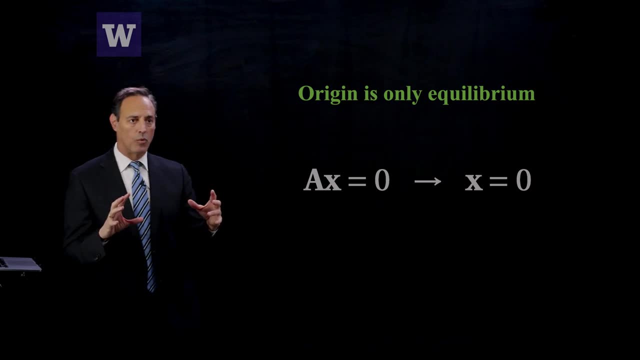 looking at currently non-singular matrices, and so we want to think about that, And, in those cases, non-singular matrices a, then, in fact, the only equilibrium point is the origin, And this is going to be part of what we focus on. 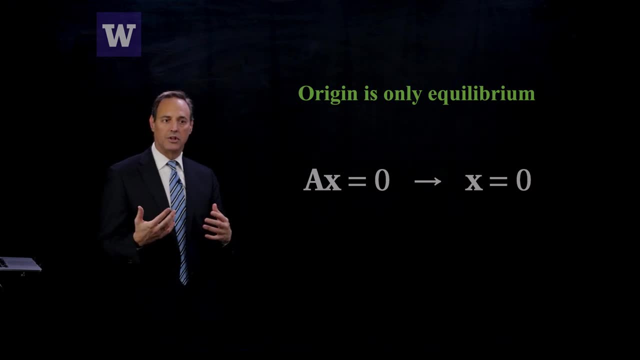 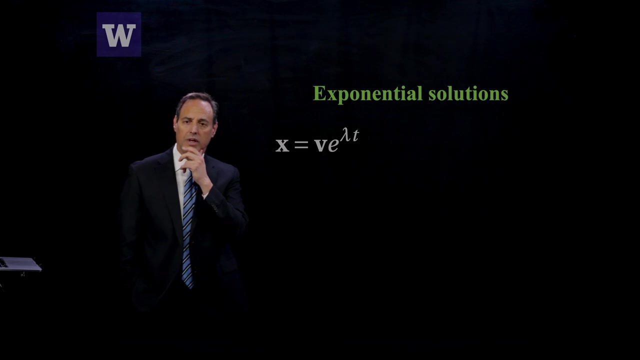 is what is behavior near the origin, which is the equilibrium point of this system? Ok, so what are the possibilities and how we're going to go solve this system? So what's standard to do in linear differential equations is to look for solutions that are exponentials. So that's just the common thing, that 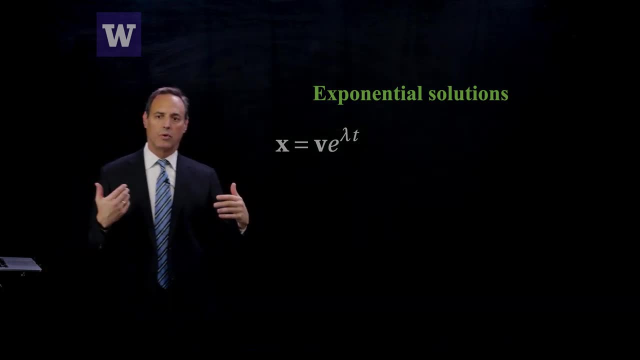 happens in looking for solutions to differential equations, linear systems, you try an exponential V equals e to lambda t. So you know what lambda is, you know what V is, and so the question is if I put in this kind of form of solution. 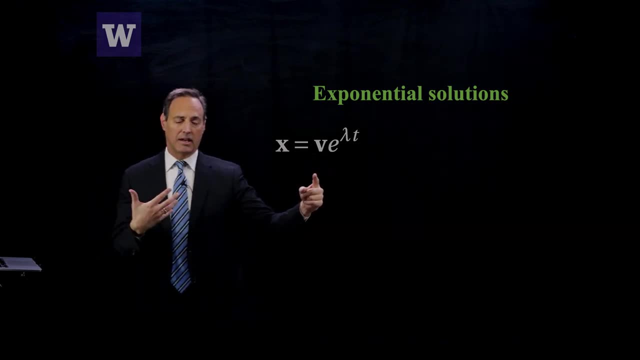 how do I find that V and that lambda that can tell me something about the types of solutions I would get out of this two-by-two system? If you plug that in what you end up with into the x, dot equals ax, you end up with a. 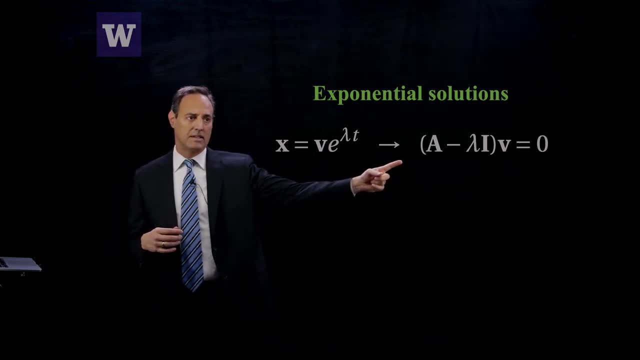 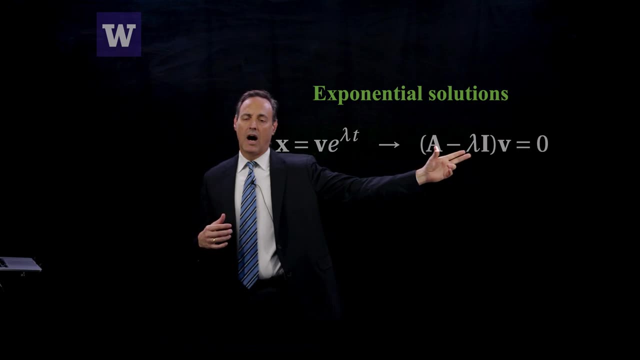 eigenvalue problem which is given right by here. a minus lambda i v equals to zero, And so what you can see right away is, if I want to solve this equation, I can look here at this: a minus lambda i, and if this actually has an. 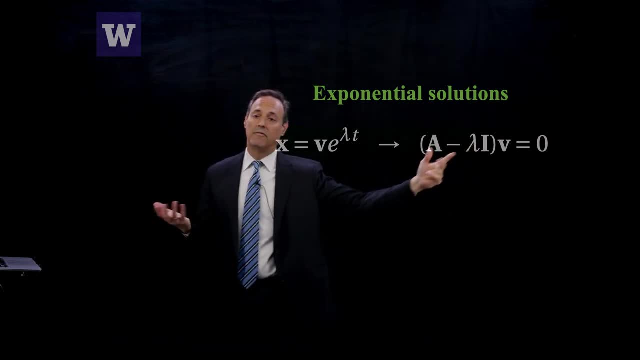 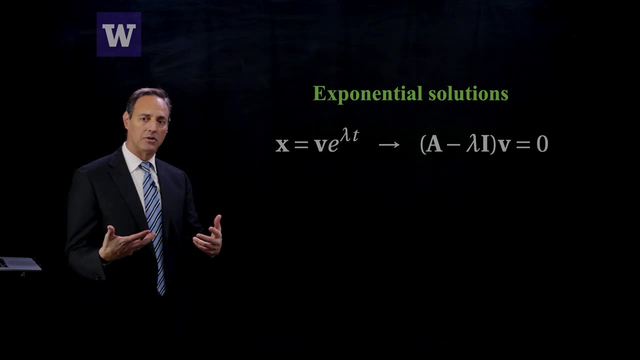 inverse, then you can take the inverse and you'll find v equals zero And v equals zero is not a very interesting solution. it's the trivial solution and I want to find non-trivial solutions to this problem. Another possibility is to pick the lambda. 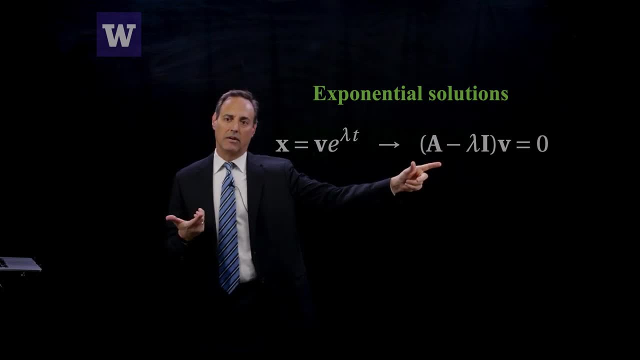 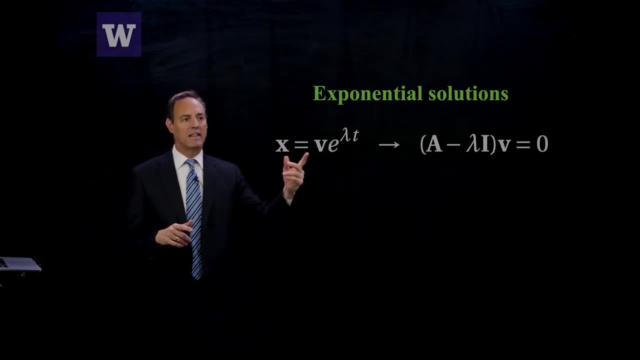 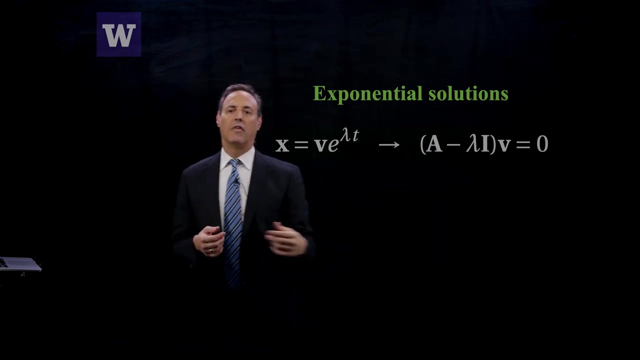 to make this a minus lambda i singular, And in that case there is the possibility of being able to write down solutions and in fact, those values that make that a minus lambda i singular are called the eigenvalues and the corresponding v are called the. 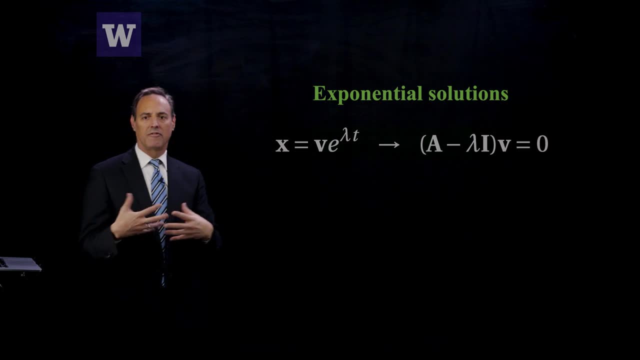 eigenvectors. Okay, so this is just an eigenvalue, eigenvector decomposition by trying exponential solutions to this linear differential equation. And that's the standard thing you would do with any linear differential equation is just try an exponential solution. Okay, and, by the way, the exponential solution isn't just 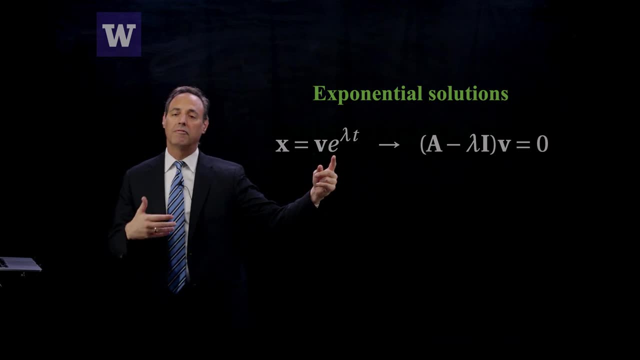 depending upon what lambda is, if it's real or imaginary, you can get very different types of behavior, whether it's growth or decay or oscillations, And in fact, this form of solution there's only unless the eigenvalues are purely 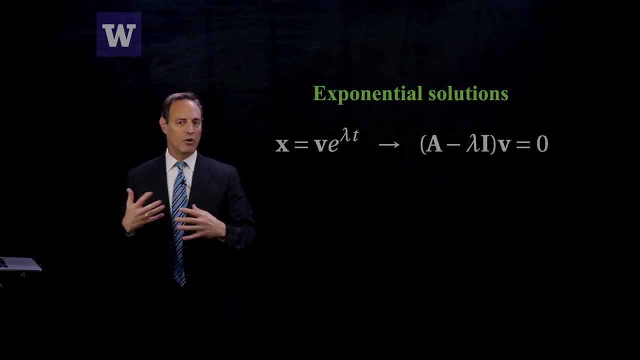 imaginary, all the solutions are either going to go to infinity or go to zero, okay, Unless you have purely imaginary lambda values. So that's something to keep in mind as you start thinking about the types of solutions you want to get out of this. 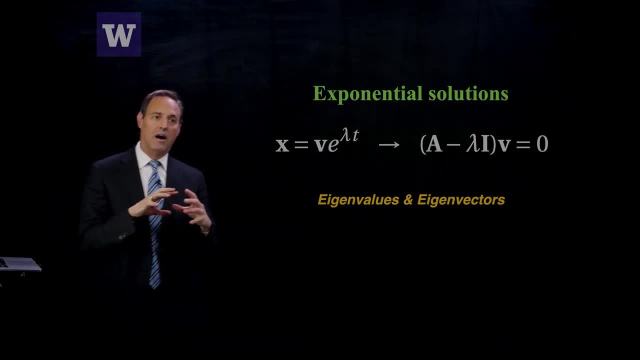 So the eigenvalues, eigenvectors of the matrix A are gonna determine all the behavior, the final, the final function of a matrix A are gonna determine all the behavior, the final function of a matrix A, the behavior for us in these systems, And so it's important to calculate those. So, and in fact, 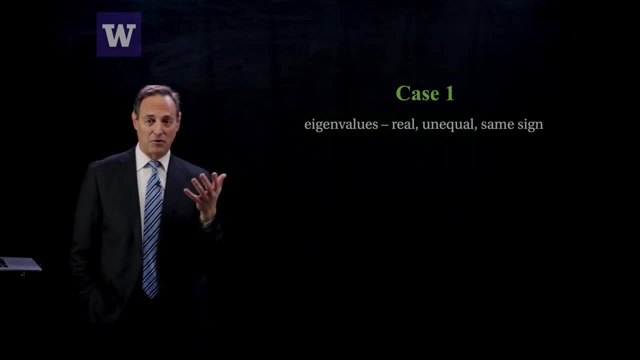 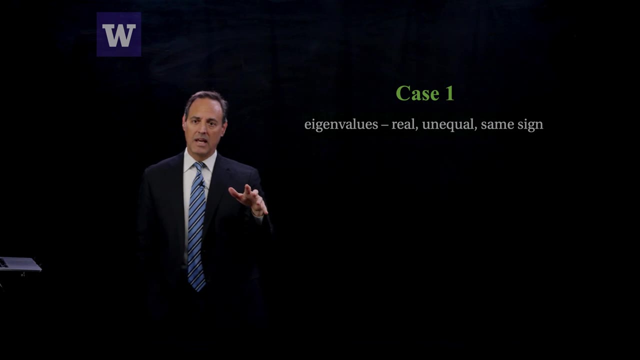 what I really want to do is, I'm assuming you know how to calculate eigenvectors and eigenvalues of a two-by-two system, but really what you want to do is highlight the different types of behaviors you can get in this system, And there's five canonical cases and I want to walk through those. 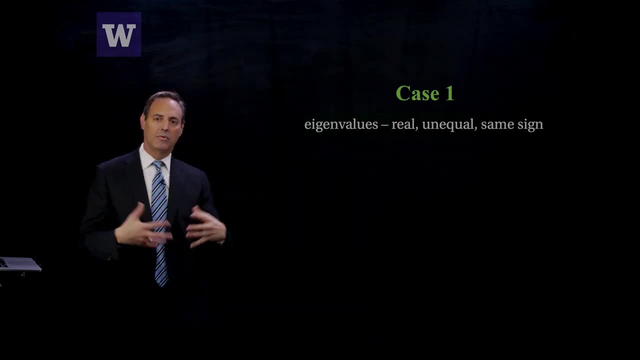 because in many ways they're going to set up the basis for us to understand a much richer set of dynamics when we go to nonlinear systems- because nonlinear systems are going to be made out of components, out of the linear systems- At least our qualitative understanding of that will happen. 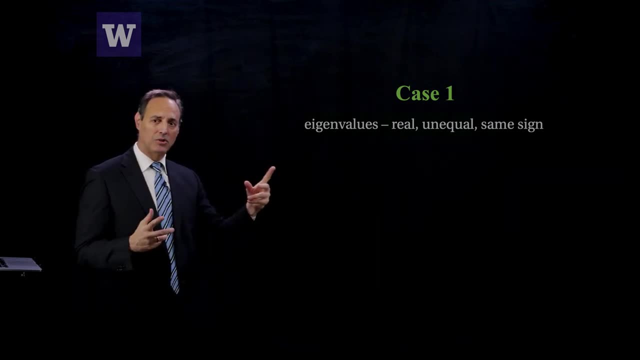 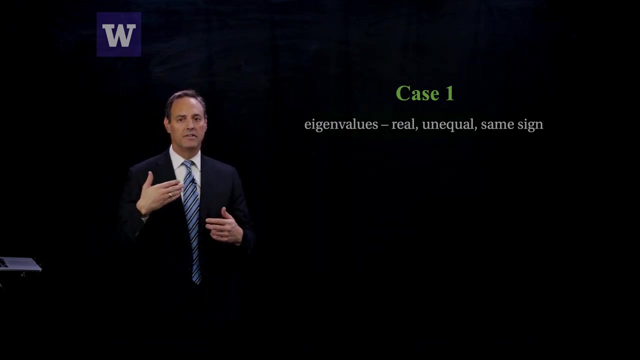 through linear systems. So let's look at this Case one. The eigenvalues are real, unequal and are the same sign, So they can both be positive or both be negatives. okay, And if we have that, what we can find is for each one of those eigenvalues there is a corresponding eigenvector. 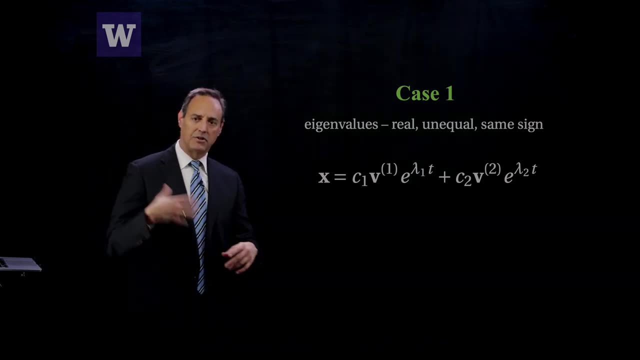 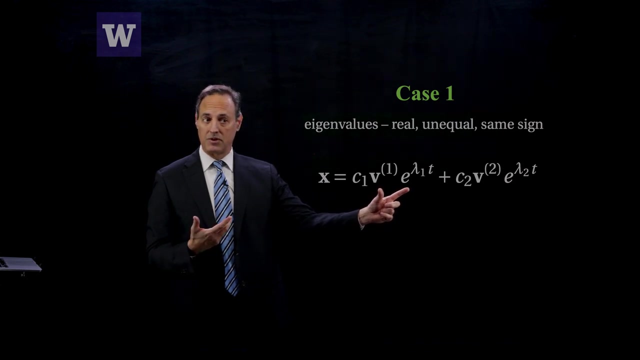 So generically, our solution is going to look something like this: It's going to be a linear combination. So since it's a linear system, we can rely on linear superposition for this solution type, which is one solution here: V1, eigenvector V1 times eta lambda 1 t. the solution V2- eta- lambda 2 t. 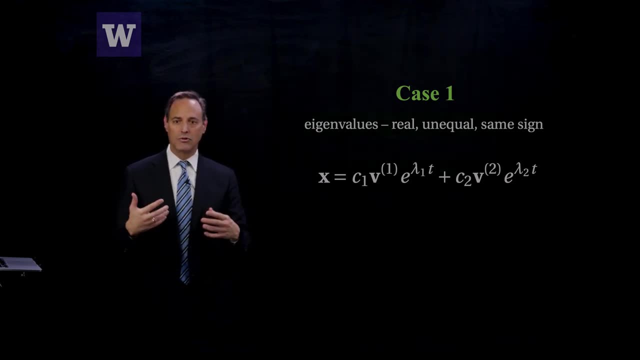 So you just add these together, You can determine C1 and C2 based upon the initial conditions of your problem, and then you can analyze the solution. Now notice that, depending on lambda 1 and lambda 2, if they're both real and positive, right then the solutions. 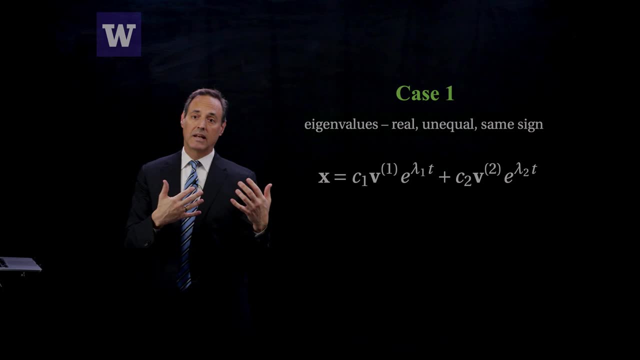 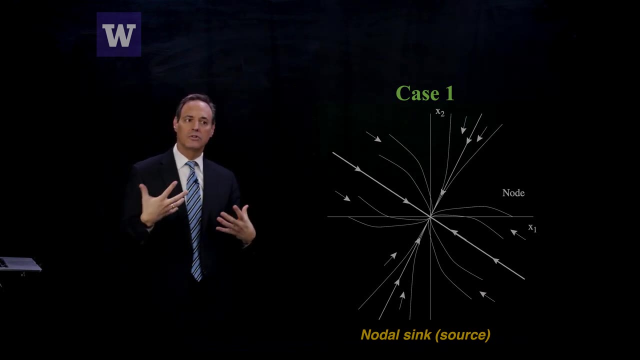 are going to blow up exponentially. If they're both real and negative, then the solutions are going to go to zero. okay, And the generic way to construct what this solution looks like is to draw something like this. This is called the phase plane for this node, or source sink. 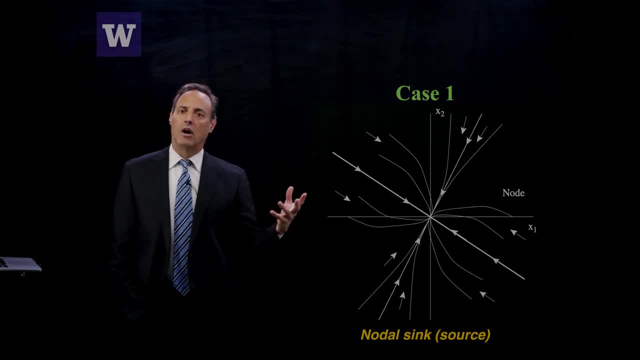 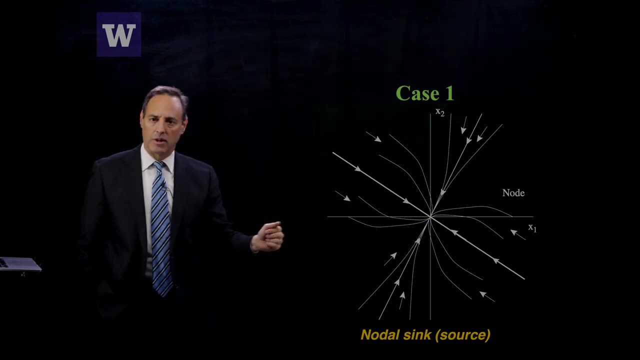 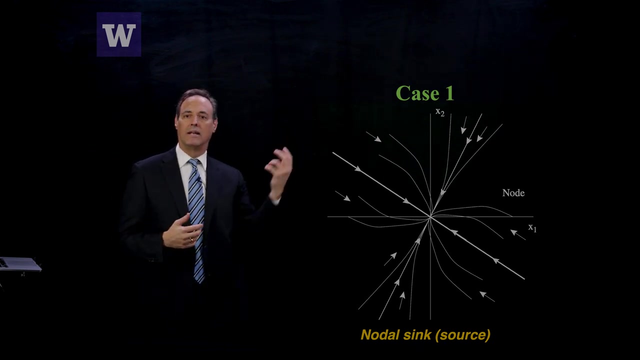 So what I've shown you here is when the two eigenvalues are real and negative. So the boldest solid lines are, let's say, the directions of the V1 and V2.. In other words the two eigenvector directions, And along those eigenvector directions you have a decay of lambda 1 and a decay of lambda. 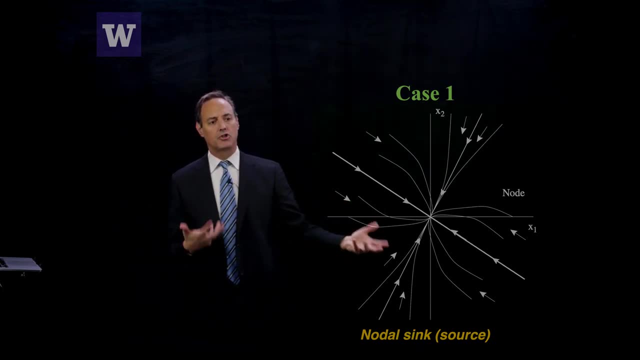 2. And so you generically get this kind of structure here, which is everything is going to the origin and it's going faster along one direction than the other. In fact, it's going faster depending upon which one is: lambda 1 bigger than lambda 2, or vice versa. The biggest one tells: 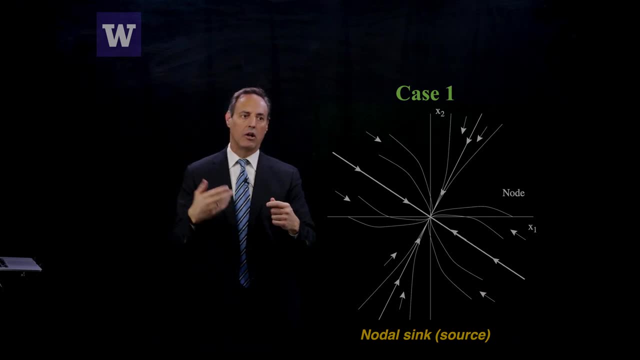 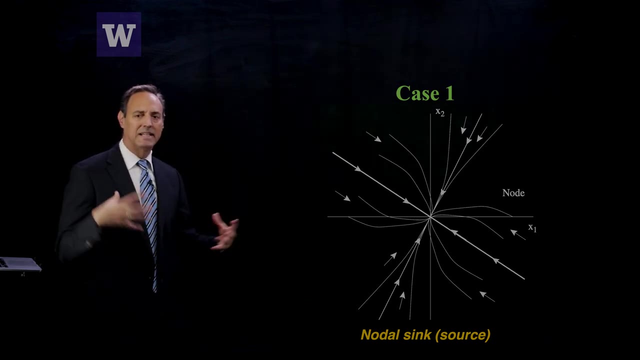 you the fastest decay rate, So it's decaying faster along one direction than the other, So it's decaying more quickly along one direction than another. And then you get this kind of structure here. okay, What I've drawn here is a sink. All the solutions go to zero If the eigenvalues were. 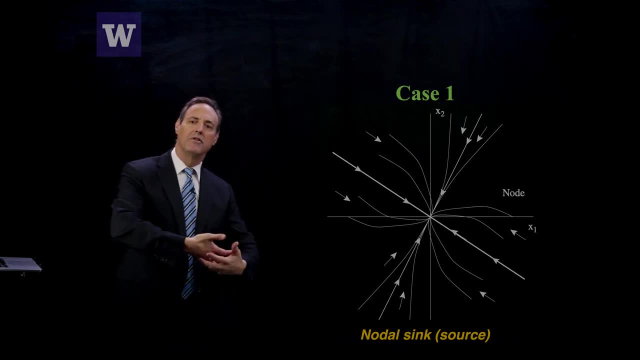 both positive, all those arrows would reverse their direction. Everything would be going out to infinity and that would be called a source. So again, this is the canonical picture for the eigenvalues and eigenvector system, when the two eigenvalues are both real and negative. 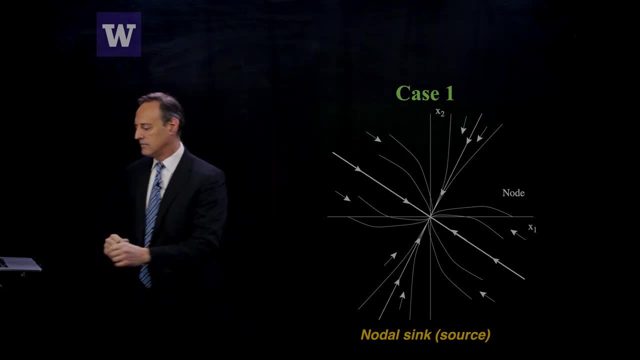 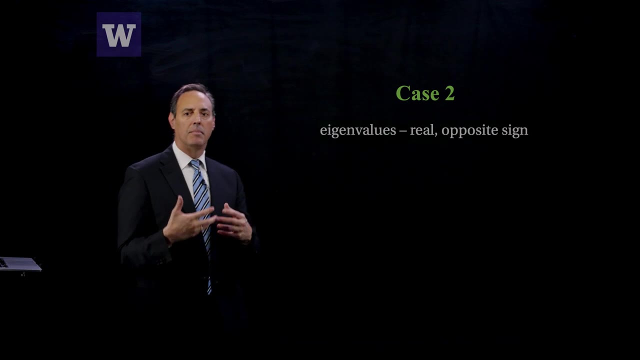 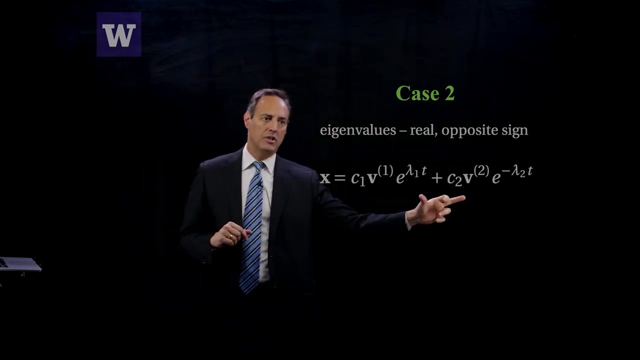 So that's case one. Case two is we can again consider real eigenvalues, but this time the eigenvalues are opposite sign, One is positive, one is negative. So the generic solution type is going to look something like this: Lambda 1t e to the minus lambda 2t. So this is going to be. 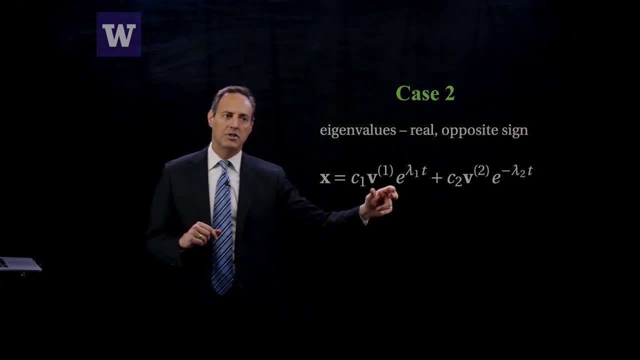 our solution type right here. okay, And you can see one of them. let's say that if lambda 1 is positive, then this one here is growing exponentially, so the solutions go to infinity, While this one here, if lambda 2 is positive, then the solutions are decaying and 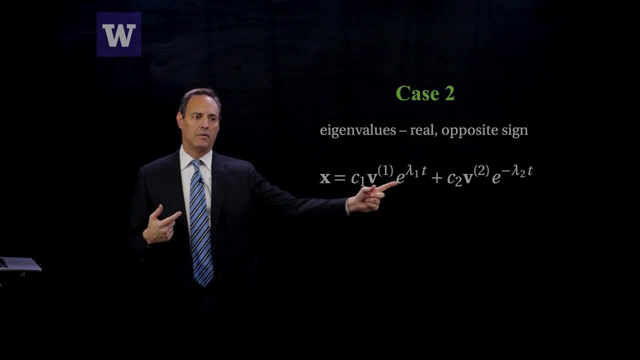 going to zero. So you have one stable direction, which is along this eigenvector here, and you have an unstable direction along here. What I mean by stable or unstable is: do solutions go to zero or do solutions go to infinity? All those solutions that go to infinity. 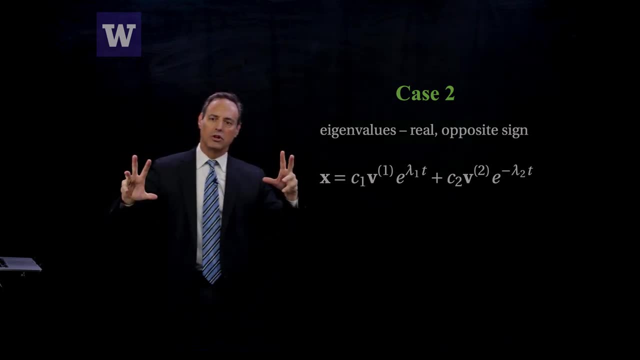 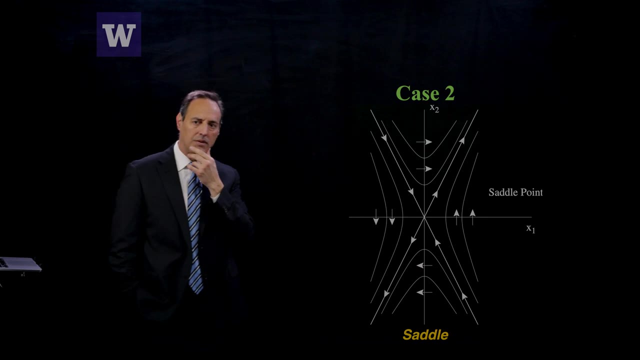 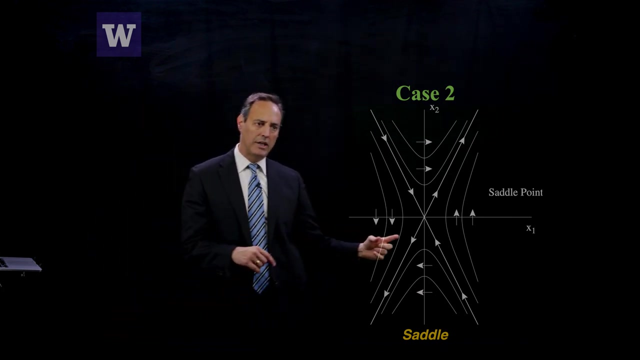 they blow up. those are the unstable solutions, and all the solutions that go to zero are the stable. So that's the generic structure and this is kind of what the sort of prototype look of case two looks like. It's called a saddle, In other words, you have directions here and what I've drawn here. 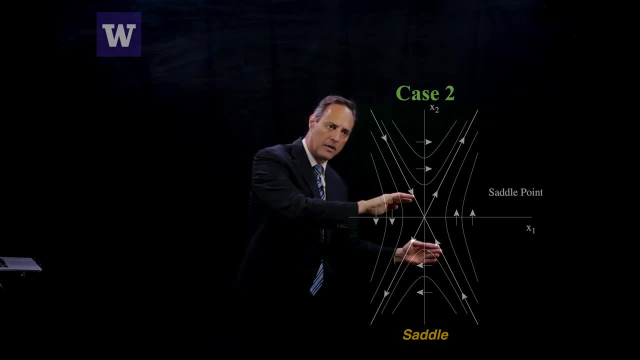 is along these two directions, right here, right here, these are the eigenvectors that are decaying exponentially in towards the origin and along these directions, here is them exponentially growing away from the origin. okay, So you come in along one direction and go out. 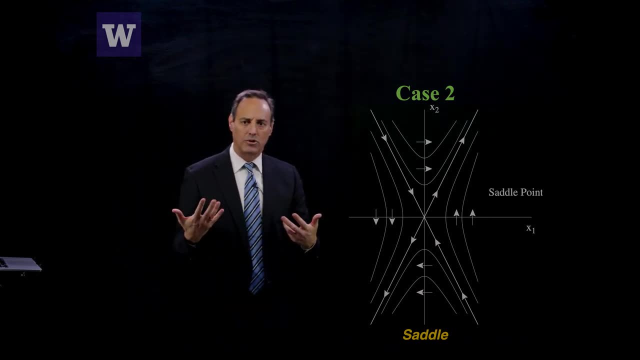 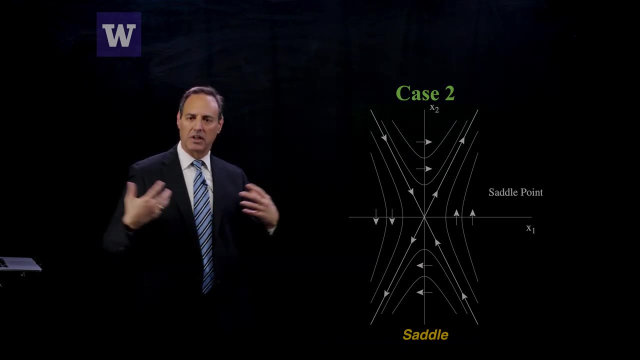 along another. This saddle structure is a very important structure. It shows up in many systems and in fact it's a sort of a canonical, interesting case of dynamics that get attracted near a point and then go off, fly away from that point, and that's the state saddle and the saddle is 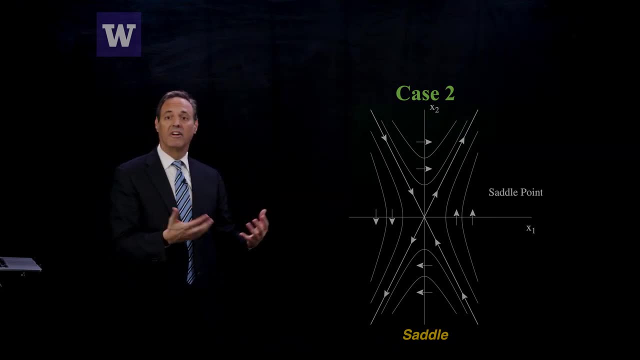 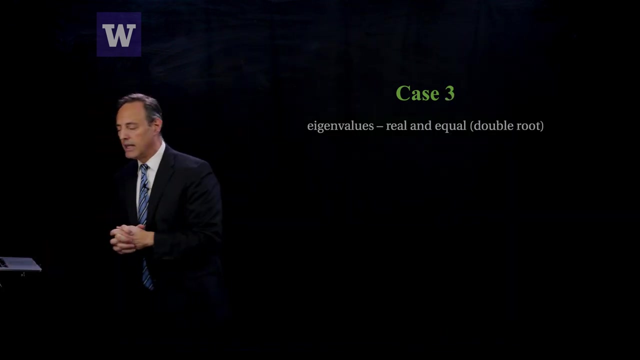 considered unstable because all the solutions eventually move away from it. even though it's initially they might come toward that fixed point or the equilibrium point, eventually they get ejected out towards infinity. So that's case two. Case three is again the last case we're going to. 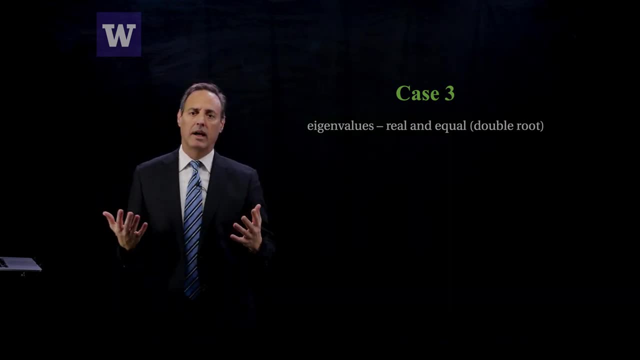 consider with real eigenvalues. but suppose those two eigenvalues are in fact identical, In other words it's a double root. So you find these eigenvalues and you get a double root, and double roots or, you know, multiple roots of a system are very 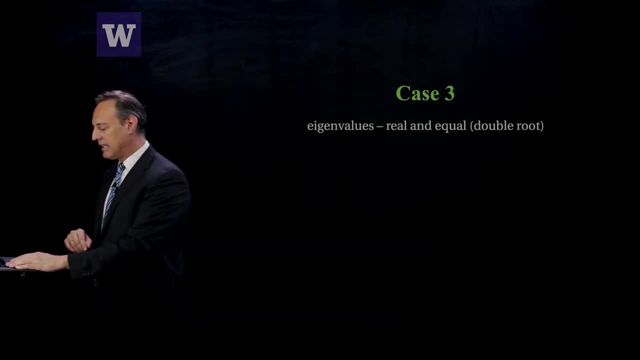 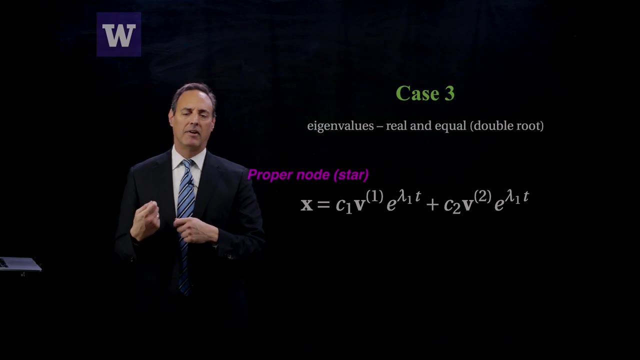 interesting. We won't talk about them too much right now, but it does give you two possibilities. One possibility is that when you find this double root, you actually go back to find your eigenvectors and you find two distinct eigenvectors. So for one single eigenvalue you'd get a v1, and you'd get a. 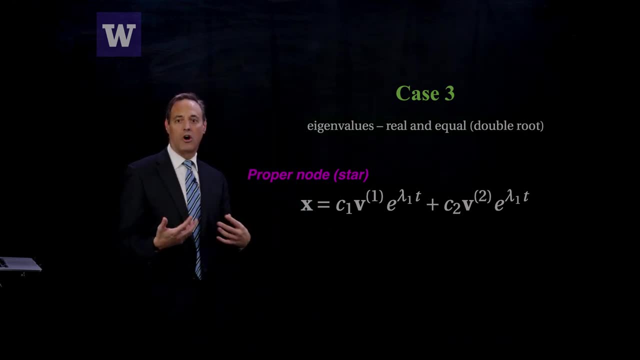 v2.. This is called a proper node or a star. In other words, there's no preferential direction, either as a source or a sink in which the, the, the, the dynamics is flowing faster, And so you just have these two directions and you get this with. like I said, 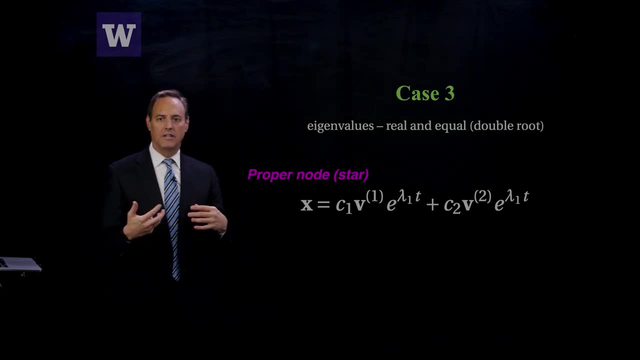 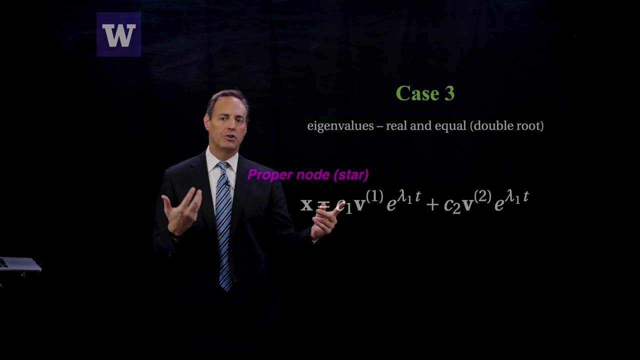 proper node or a star. However, often is the case that you cannot find two linearly in two different v1 and v2, okay, And so what you're going to have to do is find what's called a generalized eigenvector or an improper node. 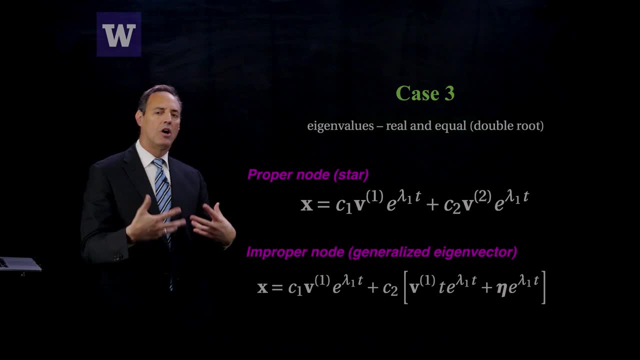 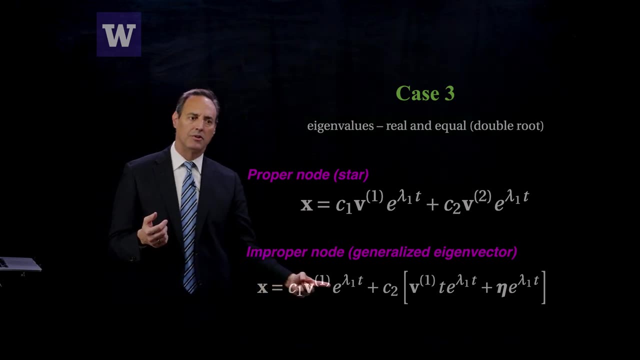 And the improper node is very much, takes on the form of the first eigenvector. So here's the first eigenvector v1, along the e to lambda 1t direction. but the improper node tends to give you a solution that where you have 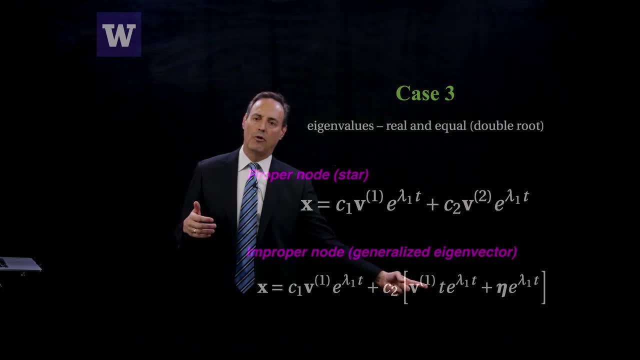 te to the lambda 1t. So it picks up this polynomial expression in front of this eigenvector. In fact, if you have a higher multiplicity of eigenvalues, in other words if you are in a higher order system of linear first order equations, 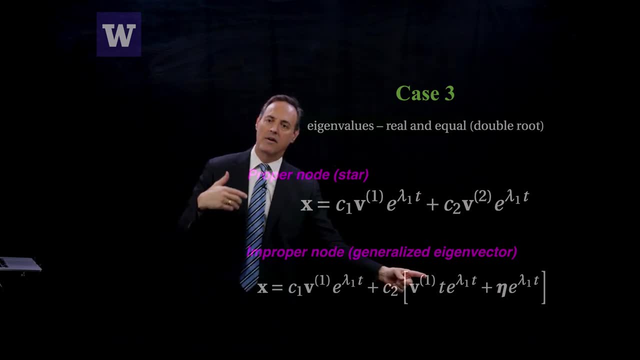 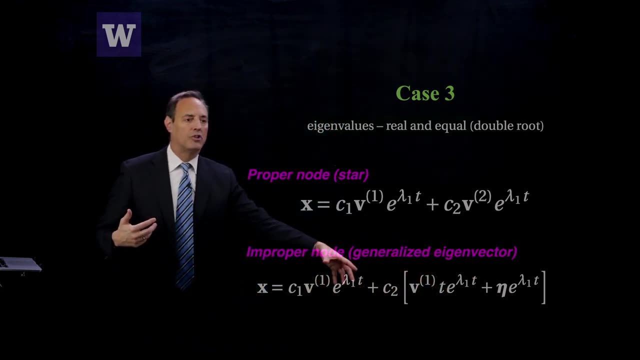 and you say you had a triple root, you might have a t squared e to the lambda 1t and so forth, Plus some generic vector eta e to the lambda 1t. So this is now what's called a generalized eigenvector for this double root case. 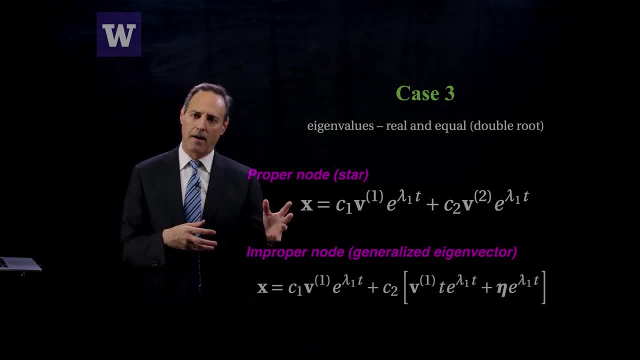 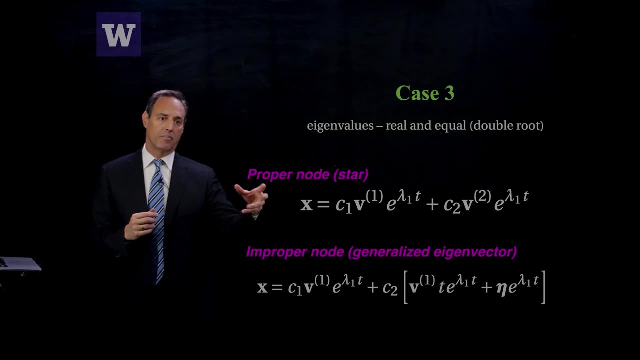 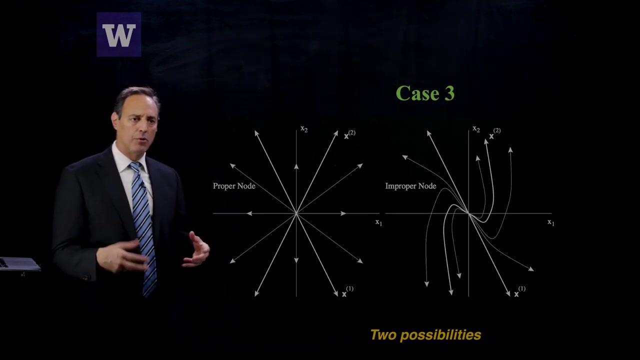 And so there's two. those are the two possibilities you have when you have double roots or multiple roots in general is that you have to decide if it's a proper node or an improper node. okay, And this is what these look like. In the proper node case, you have these two different eigenvectors. 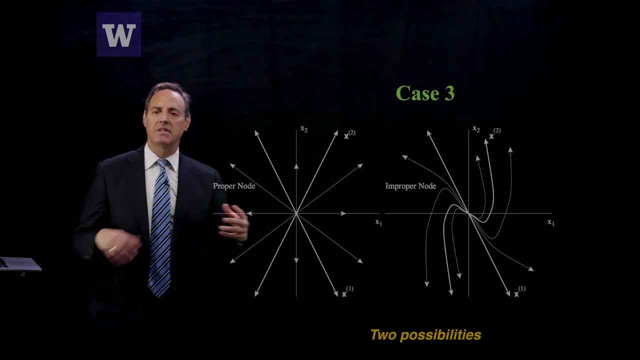 V1 and V2 represented here, but since everything's either growing in the same direction or decaying in the same direction, it just looks like a star. Everything is equal direction. everything goes out, flows out of that equilibrium point or comes into the equilibrium point at the same speed in every direction. 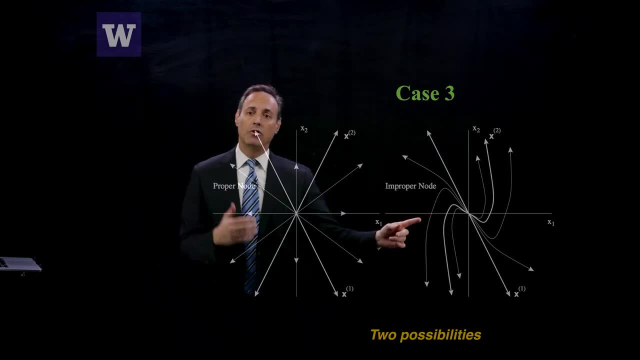 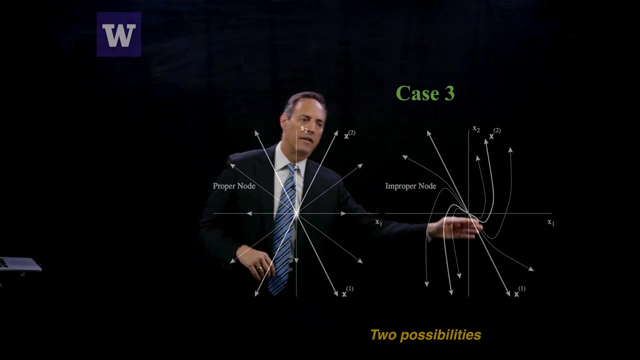 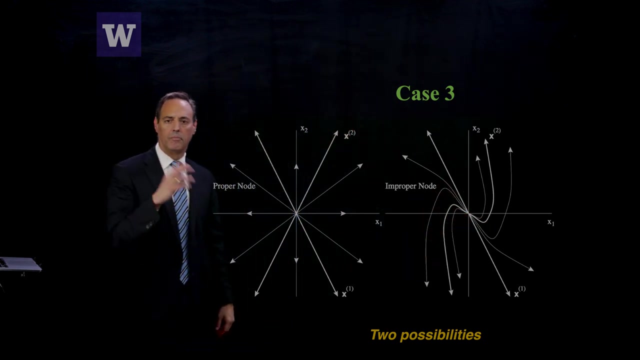 In case of an improper node, you find this generalized eigenvector in which look at your structure of your eigenvectors. They actually have shapes to them, They're not just straight lines. So this main line here is the one eigenvector that you have, and this one here is this generalized eigenvector which we computed previously. 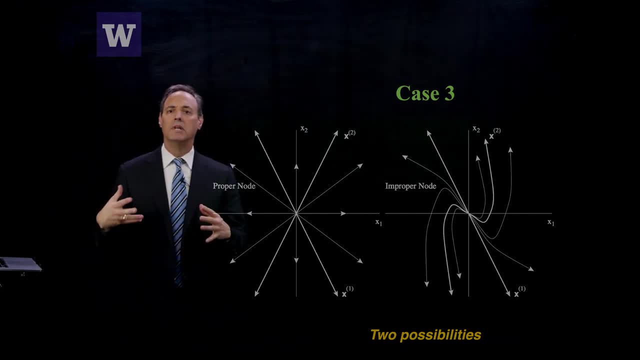 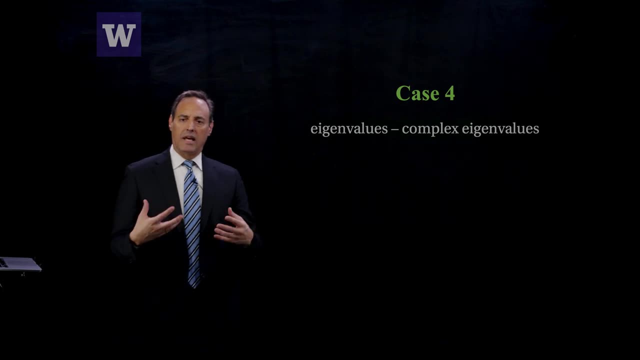 So those are the possibilities you have when you have double roots. We now move on to the case when you have complex eigenvalues, In other words, eigenvalues that are complex, They're not just straight lines, they're not just straight lines. 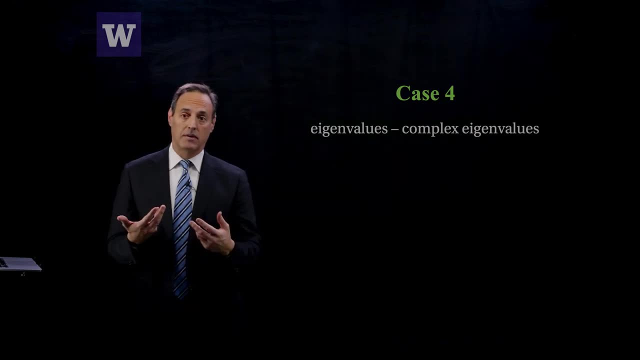 They're eigenvalues that have imaginary components. okay, So this would just come from solving for your eigenvectors and eigenvalues, and the way you do it, for a two-by-two system. you're actually solving a quadratic equation and that quadratic equation can produce imaginary components to the eigenvalues. 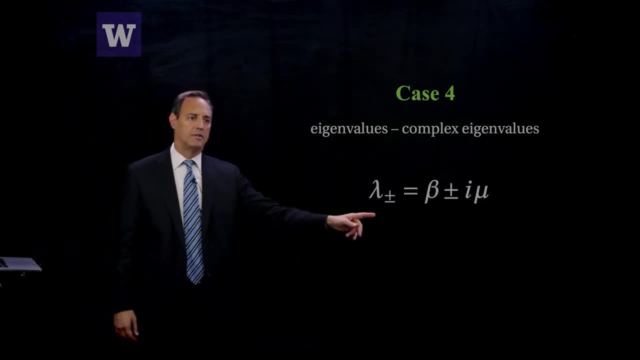 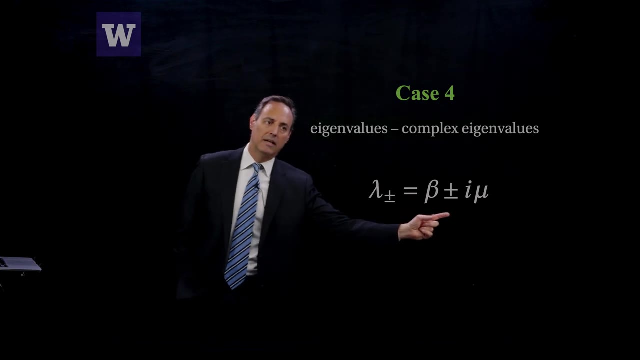 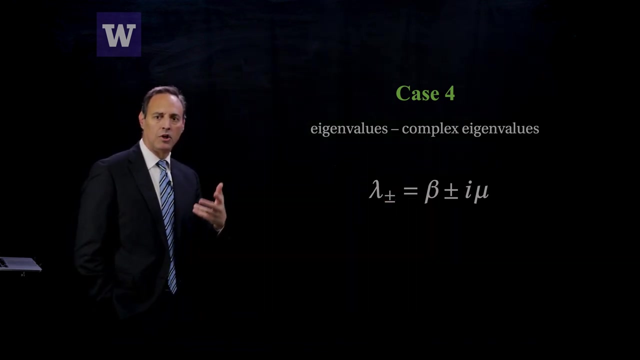 So these complex eigenvalues have a structure like this: There's a real part and a complex conjugate pair of plus or minus eigenvalues. So the real part is beta and mu is the complex piece to this. Now, beta determines whether the solutions are going to grow to infinity or decay to zero. 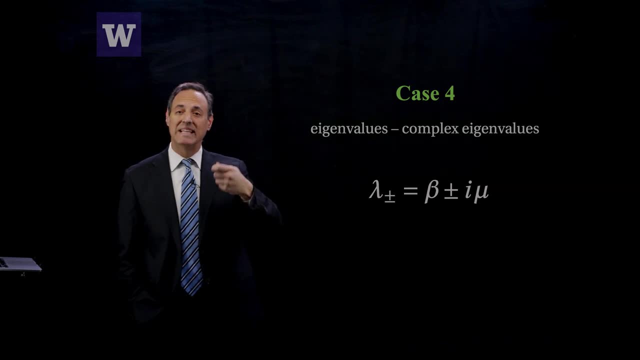 So if beta is positive, this is the real component. Remember it's e to the lambda t. So this is all being exponentiated to this real part, and the real part tells you whether you're going to get growing or decaying. 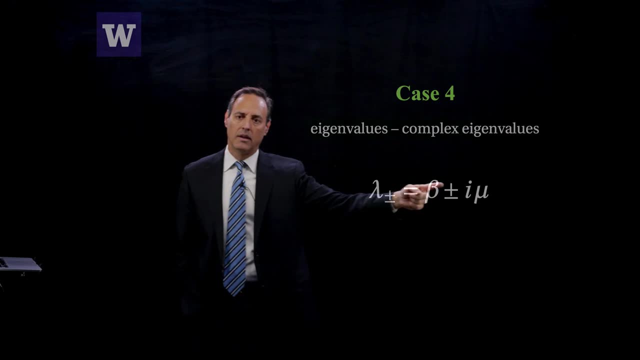 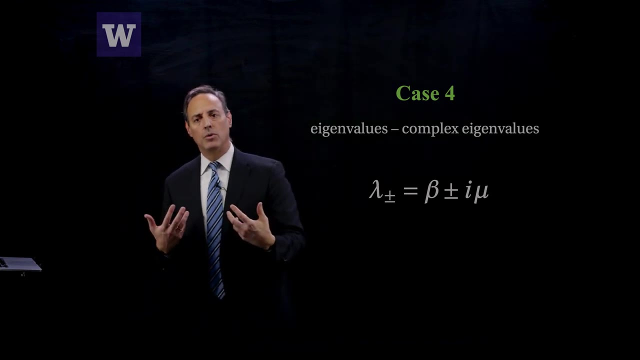 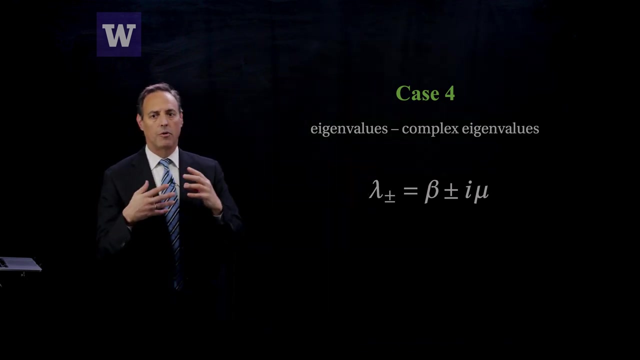 The e to the i mu t By using an Euler formula. you know that it's related to cosines and sines. So the i mu is oscillations at a frequency omega. All right, sorry, at a frequency mu. So the imaginary part of the eigenvalue tells you something about the oscillation. 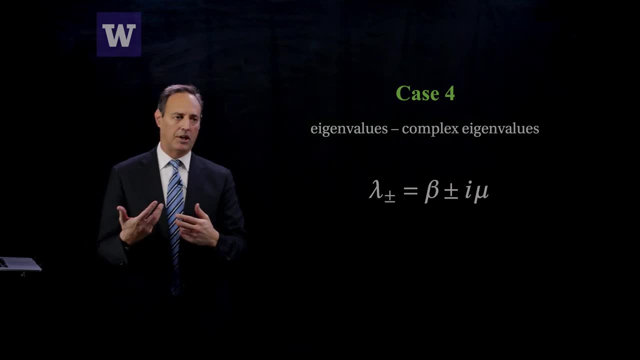 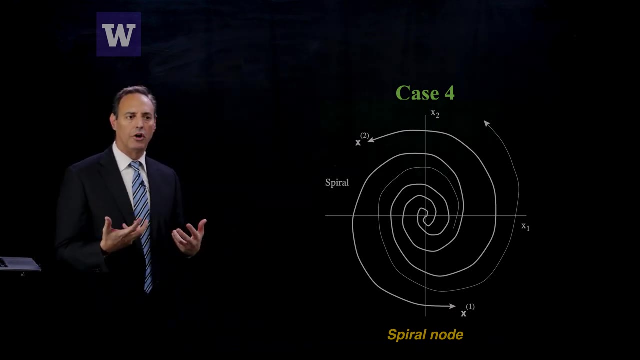 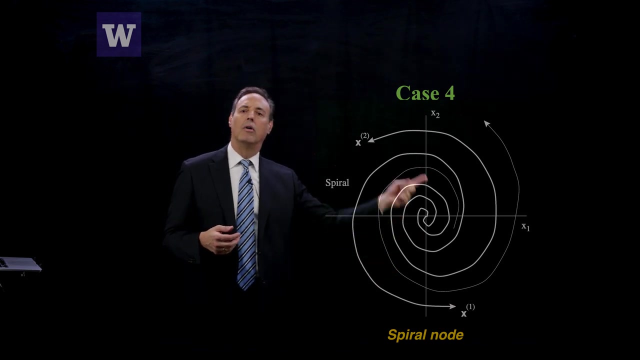 The real part tells you about growth or decay. So in general it's going to look something like this: A spiral, A spiral node, So you're going to be oscillating and growing, in this case here- And so, as you're oscillating and growing, you spiral out away from your equilibrium point. 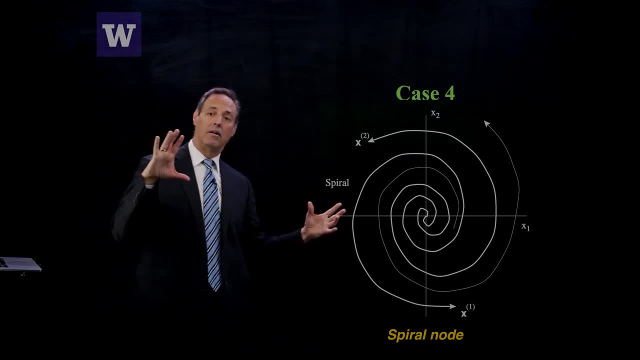 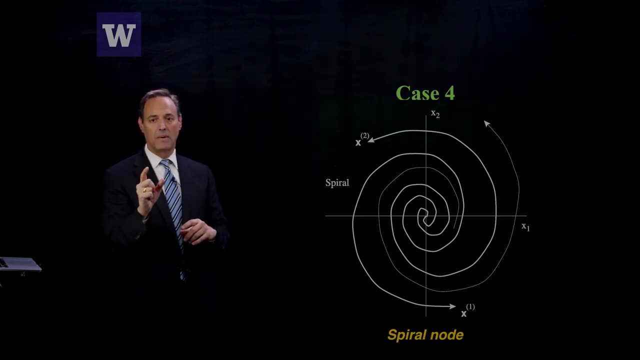 However, if beta was negative, then you'd spiral in to the origin. Okay, so those are spiral node. It's either stable or unstable, depending upon the sign of the real part. That determines everything in terms of its stability. Okay. 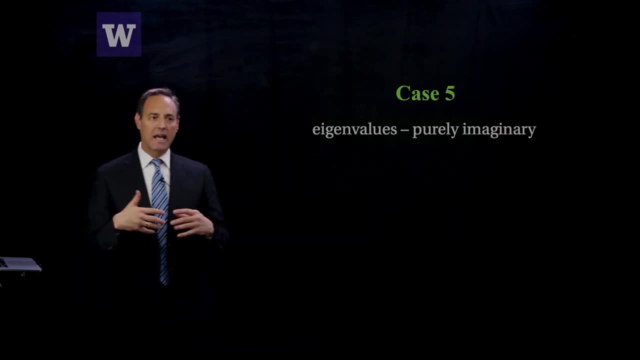 So the final case, as you might have guessed, is going to be again eigenvalues that are imaginary, but now they're purely imaginary. In other words, the real part is zero, which means you have no growth, no decay. 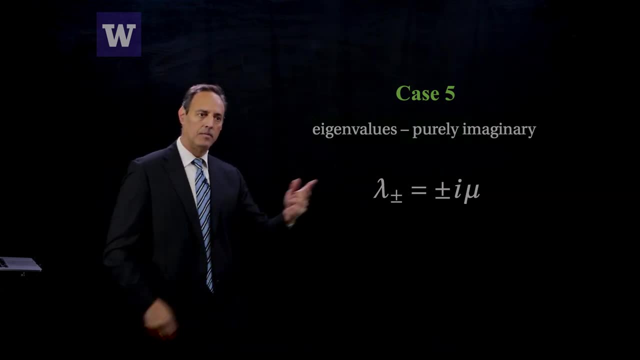 What do these look like? Well, the eigenvalues look like this: Plus or minus i mu. So you still come in complex conjugate pairs. So you have two eigenvalues, because it's a two-by-two system. They're complex conjugate pairs of each other. 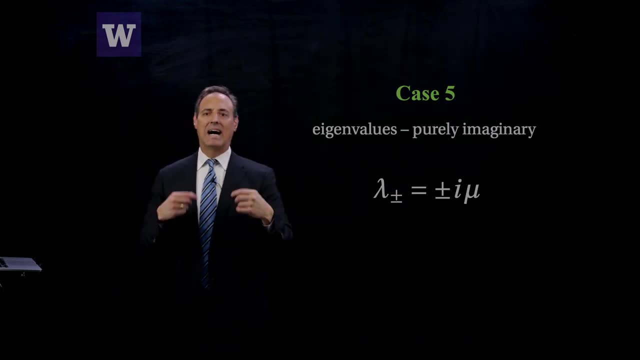 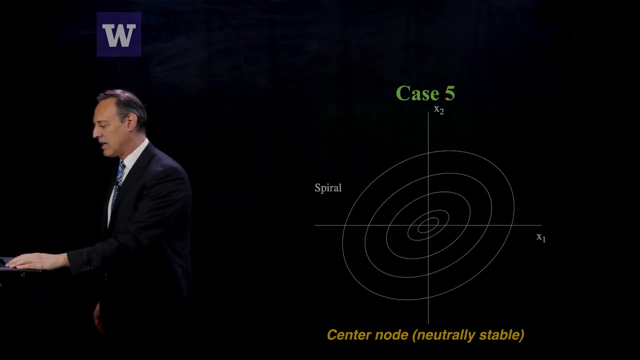 Okay, And this is going to be e to the i mu t and e to the minus i mu t, which you can express instead in terms of cosine mu t, sine mu t. So these are going to just be pure oscillations, And cosines and sines are one of our few functions that, as you go to infinity or minus infinity, they're always bounded between 1 and minus 1.. 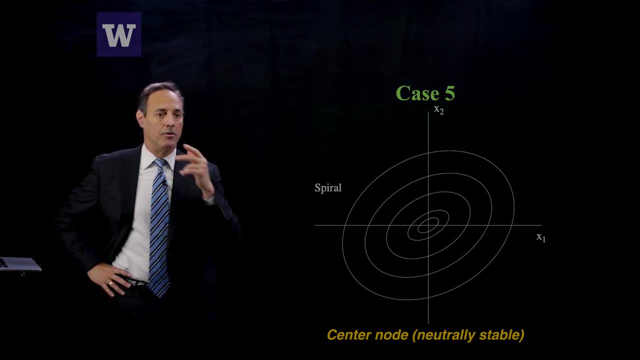 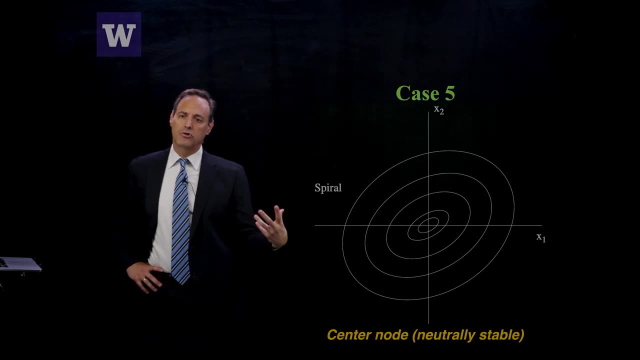 And so you get something like this case 5, which is a center node, And the center node here is just basically oscillations around that equilibrium point. So it's neutrally stable, It's not growing or decaying, And these often play an interesting role because small perturbations to this can destroy your neutral stability, which is represented here in this picture. 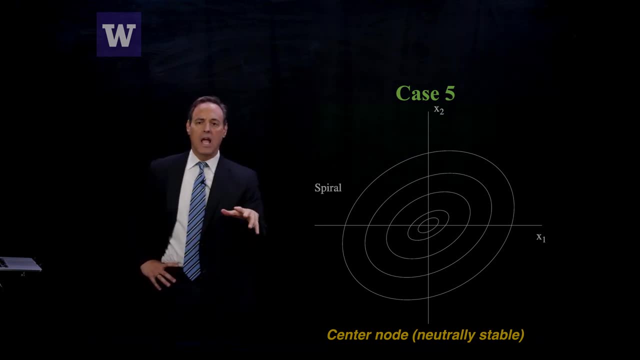 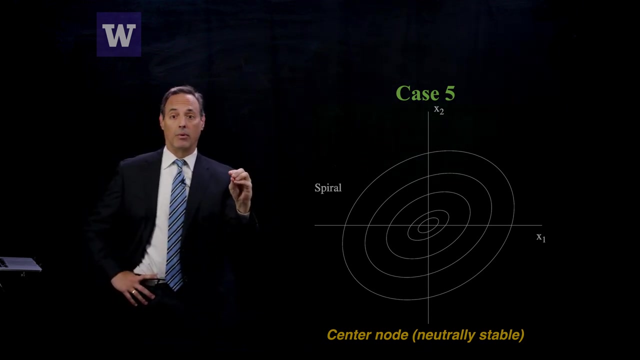 So those are the five canonical cases, And one of the reasons we're going to highlight this, at least initially for this class, is because, once we understand these five pieces, everything we're going to do in terms of start looking at nonlinear system is going to be framed locally in terms of these five behaviors, which are linear behaviors around equilibrium points. 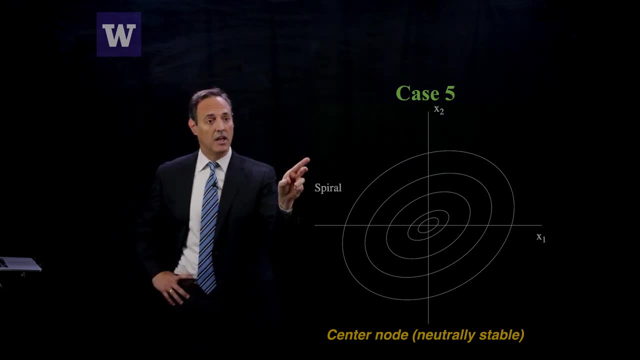 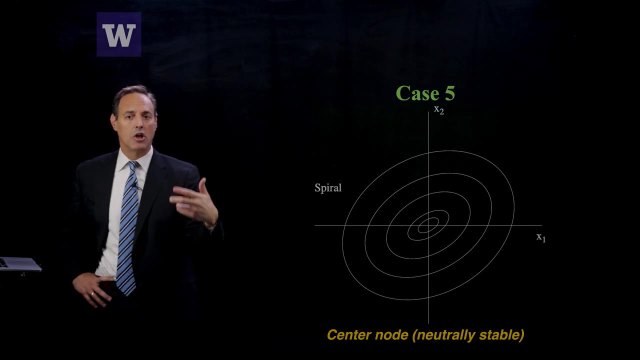 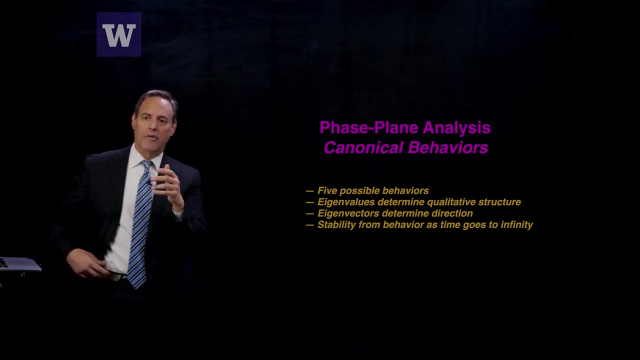 And so that's going to be the main thrust of us to try to understand: is these five cases going to keep showing up repeatedly in our efforts to try to analyze nonlinear dynamic systems? Okay, so now we're going to move on and start thinking about: okay, so this phase plane analysis comes in, these canonical behaviors. 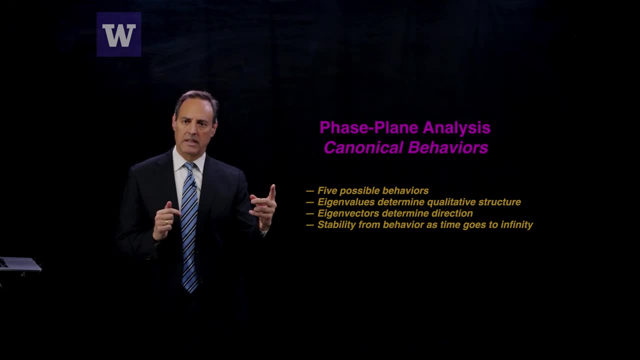 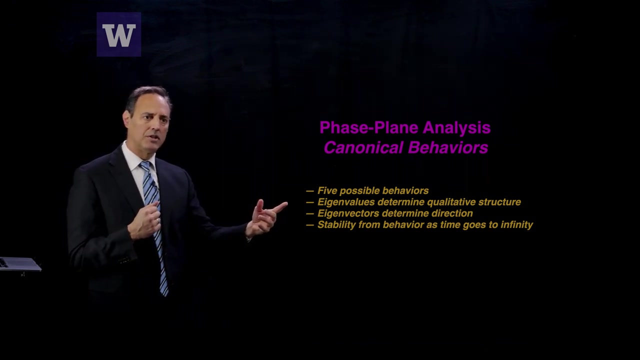 There's five possible behaviors. That's for these linear systems, And when we do our local analysis around equilibrium points, those five behaviors are going to be the prototypes for determining everything that happens in a system, And the way you understand these five behaviors is these eigenvalues. 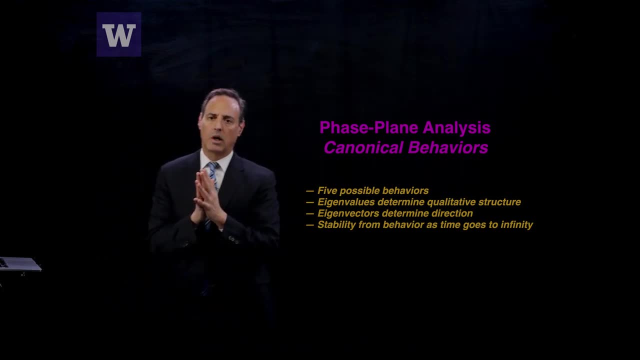 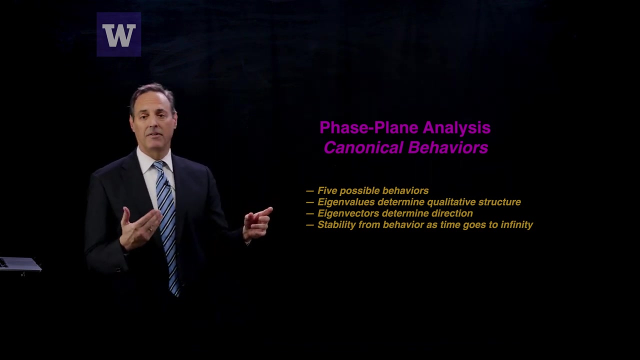 So you find these eigenvalues and that will give you the qualitative behavior near the fixed points. Whether you're growing, decaying, spiraling, these kind of different behaviors can all be deduced from the eigenvalues. The eigenvectors tell you specifically which directions in which these behaviors are happening. 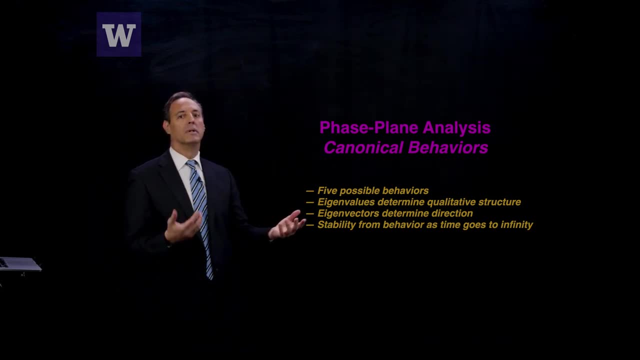 and ultimately the stability is determined just by looking at the real part of the exponential. Okay, and so that tells you if you're going to go to infinity Or go to zero. And those are the only possibilities once you have exponential solutions, unless you have purely imaginary eigenvalues in which you'll just oscillate for all time. 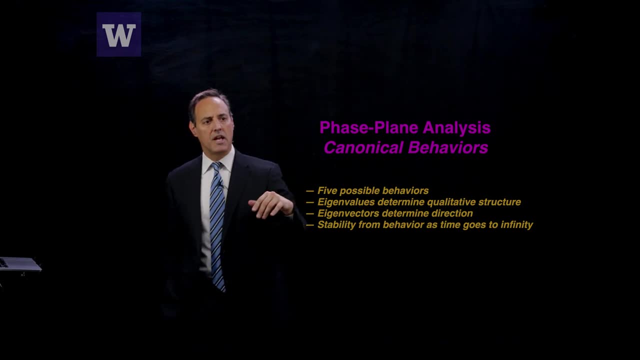 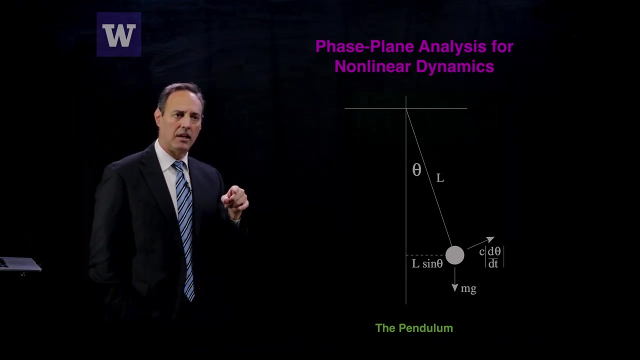 So this is an important start to understanding concepts around equilibrium and stability, and it's all framed around these five cases that I just reviewed for you here. So where I want to take this is start to come to understanding the pendulum In particular. a lot of us have studied the pendulum. 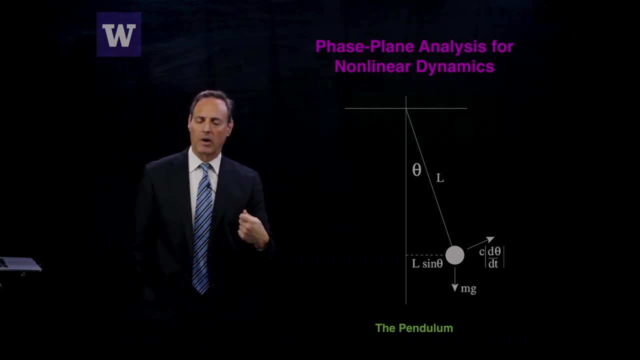 but typically we study the linearized version of the pendulum right, We look at the low amplitude or the low oscillation limit and then we can write down a much simpler equation. But we want to come here, draw this force body diagram. 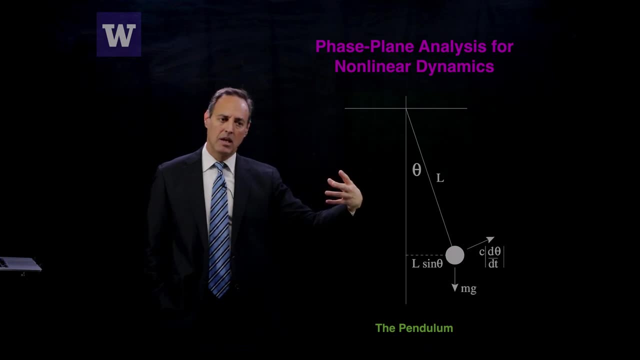 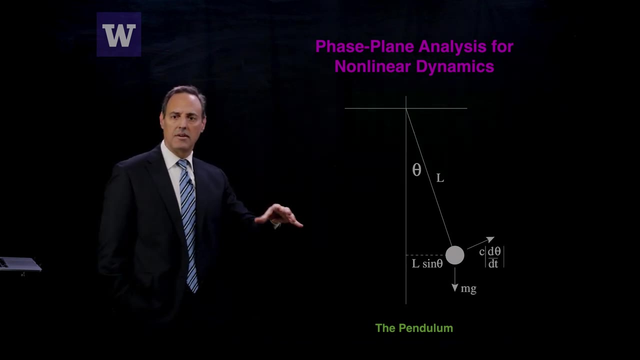 think about the variable theta characterizing this pendulum And what we want to do with it is write down the governing equations, which are nonlinear, and start to understand the pendulum in a deeper way in this phase plane analysis, Not just the linear pendulum when it's with small angle approximation. 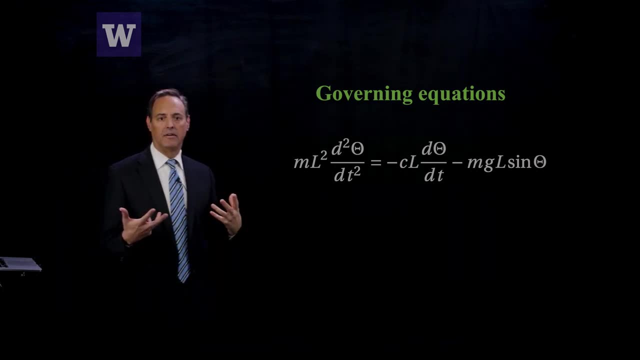 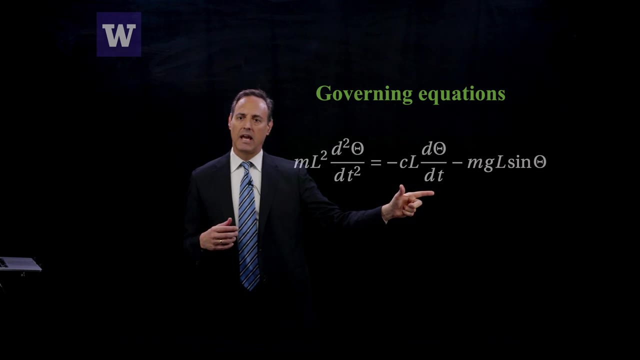 So here are the governing equations. This is just F equals ma free body diagram. What you have here is mass times acceleration here. You have here, let's say, some kind of wind resistance which is proportional to the velocity of the d theta dt. 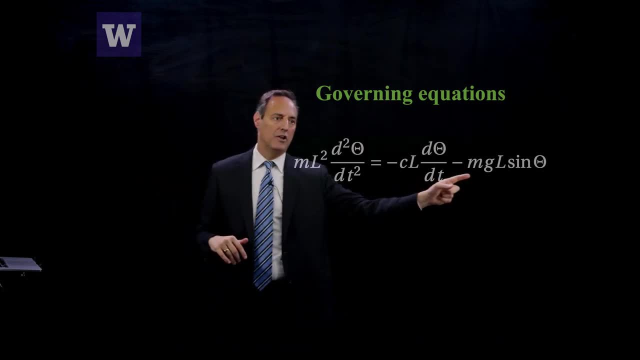 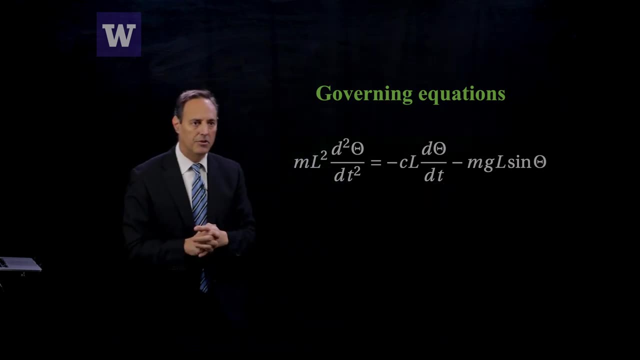 In other words how fast it's swinging, And then you have the force of gravity right here, There's the g right there and it depends upon the length of the pendulum, and so forth. So this is a classic equation, very old. 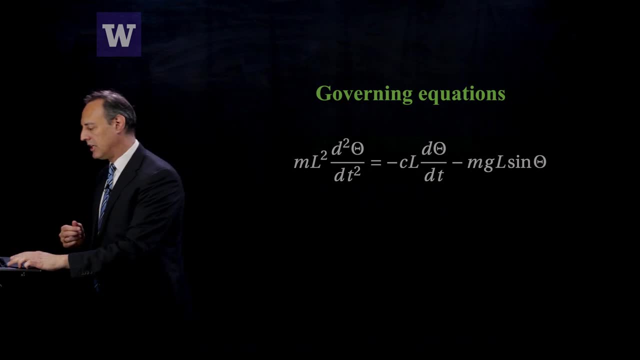 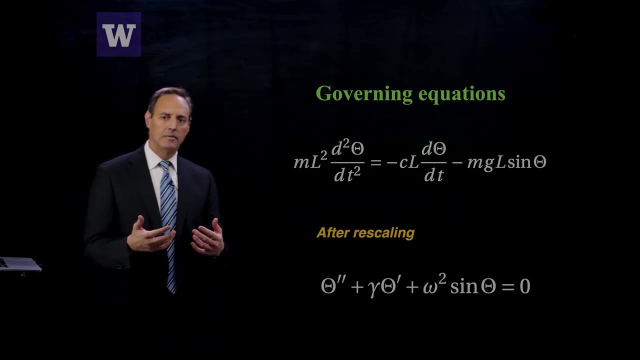 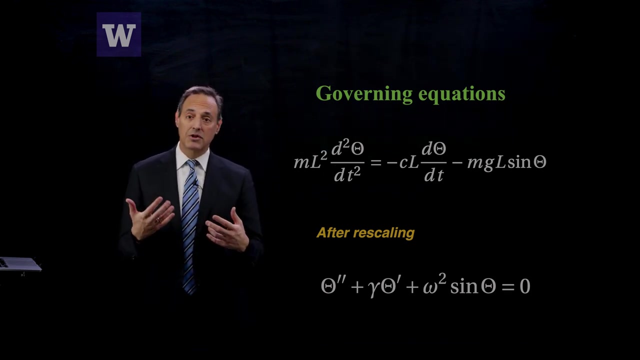 And I can rescale everything to make it a little simpler, to just write it in this form right here. So it's a second order differential equation. It's nonlinear, It's constant coefficient, And so this is a fascinating equation because the behaviors out of this 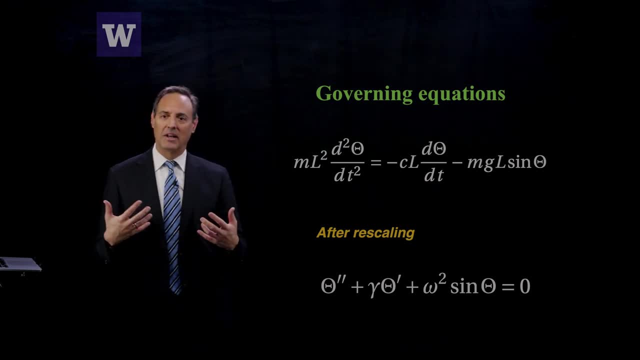 are quite remarkable and interesting, especially when you start to force this system, And we will do that later as we go through the class, But for right now we're just going to consider this base case where there's no forcing, And here's how we write it. 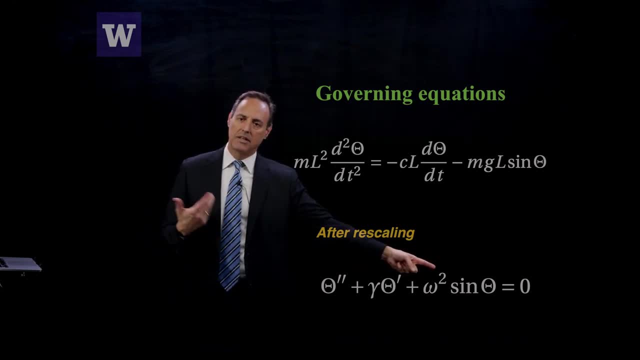 The nonlinearity is right there, the sine theta, And typically, if you've studied the pendulum before in many mechanics courses or beginning physics courses, you say that sine theta is approximately theta. That makes it linear And linear equations are much easier to solve. 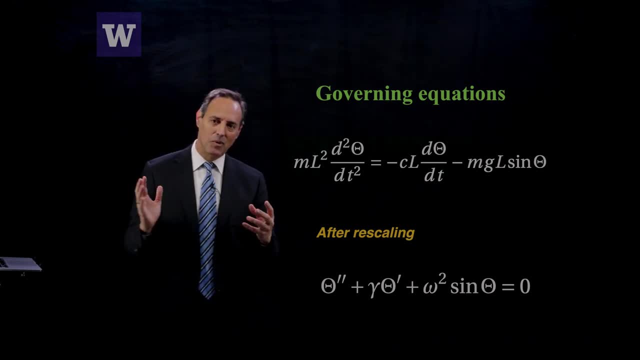 than nonlinear equations. Nonlinearity is what makes so much of life very interesting, So I want to throw that out there, because that's what this course is all about is thinking about nonlinearity both in terms of time-dependent problems and boundary value problems. 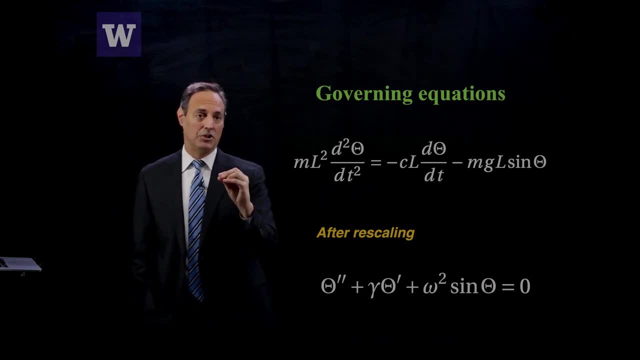 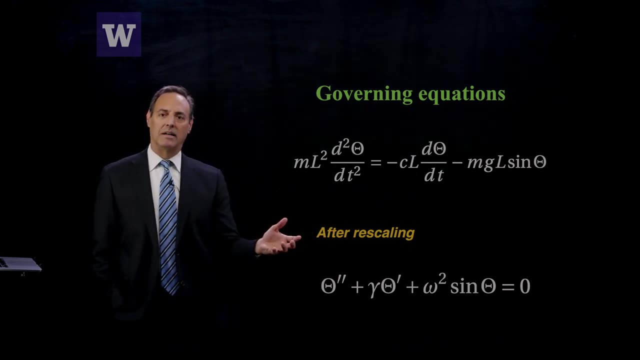 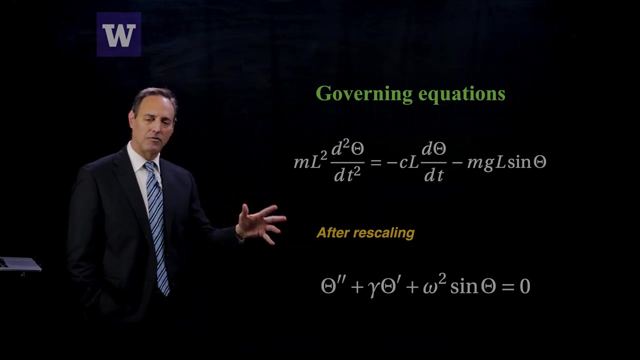 where we no longer can write down analytic solutions, but we want to make use of the fact that for linear systems that are close to it, we can write down solutions. So everything's going to be about perturbations and approximations, And we want to understand these basic cases first. 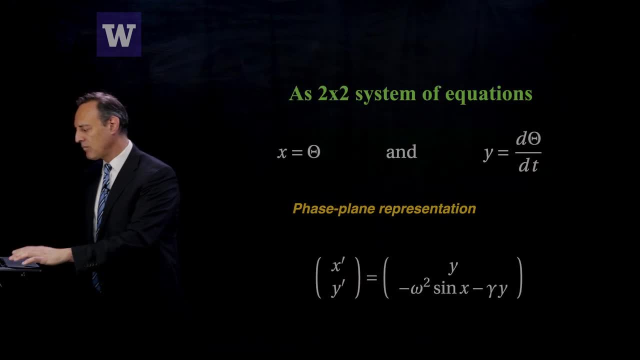 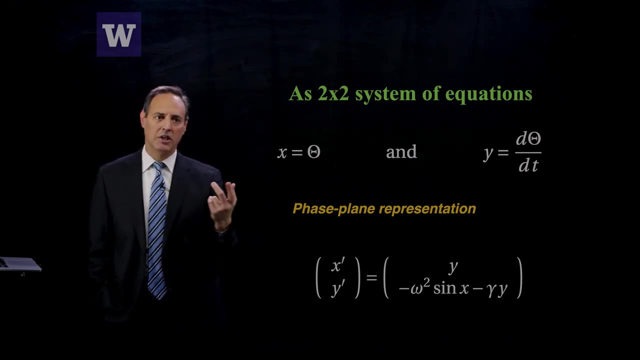 as we build intuition towards this. So the first thing we do is we take that differential equation, second order, and we write it as a system of first-order equations. So you set: x is equal to theta, y is equal to d theta dt. 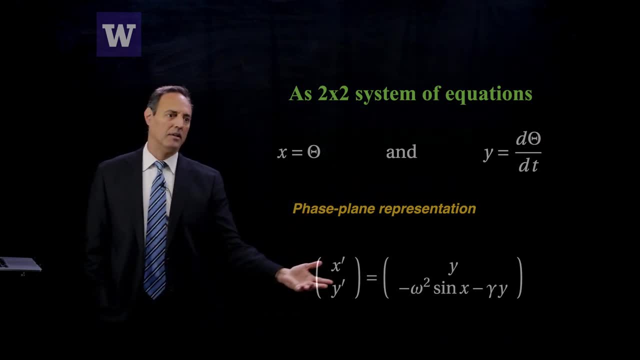 and now you have this: x dot, y dot is equal to this here. So now what I have is a 2 by 2 equation and a 2 by 2 nonlinear system of equations And the things that I want to start to look at. 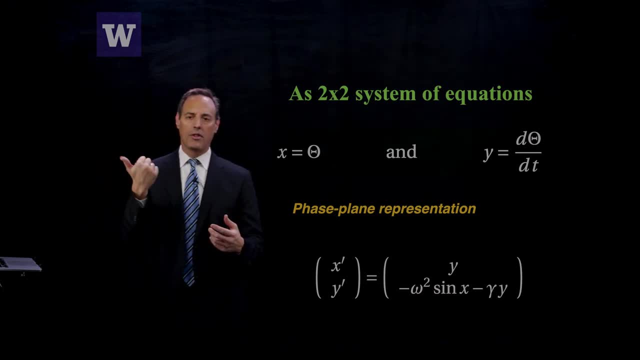 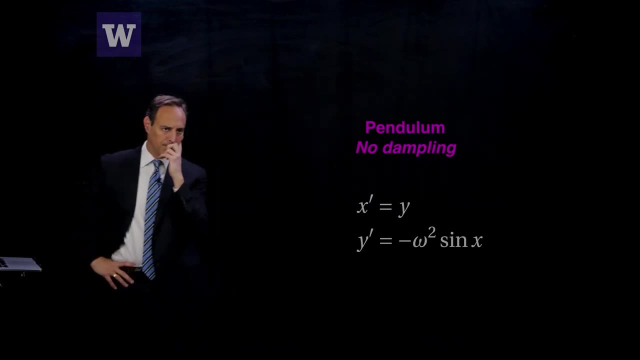 is exactly where I started with before, which is what are the equilibrium points and what are their stability. Those are the two key concepts we want to consider. So let's start off with the simplest case, or simpler case, which is the pendulum with no damping. 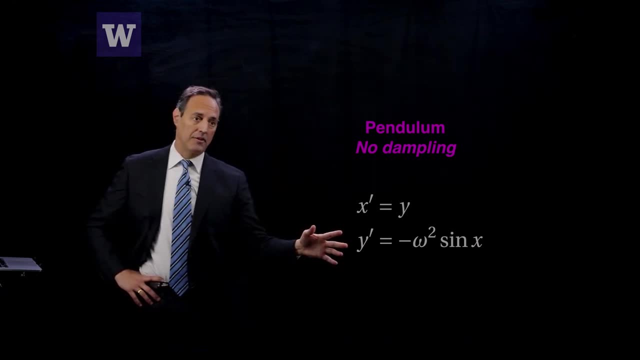 So in that case the system reduces to here. So I've taken out the damping term. so I get x dot equals y, y dot equals minus omega. squared sine x, It's still nonlinear. I've got that sine x floating around in there. 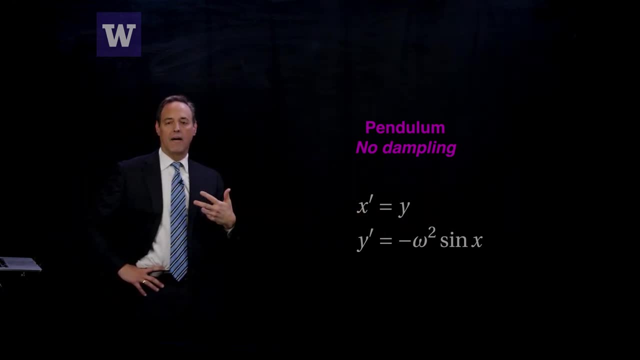 But then I can start asking: when do I have equilibrium points? Now? equilibrium points are when the solution is at rest. In other words, x dot is equal to 0, y dot is equal to 0. Well, it's pretty easy to see that x dot is going to be 0. 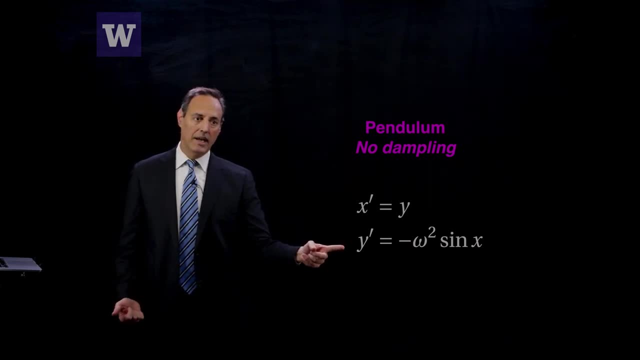 when y is 0. And y dot is going to be equal to 0, when this is equal to 0. In other words, when sine x is equal to 0. Now, sine x is 0 for any value of n pi. 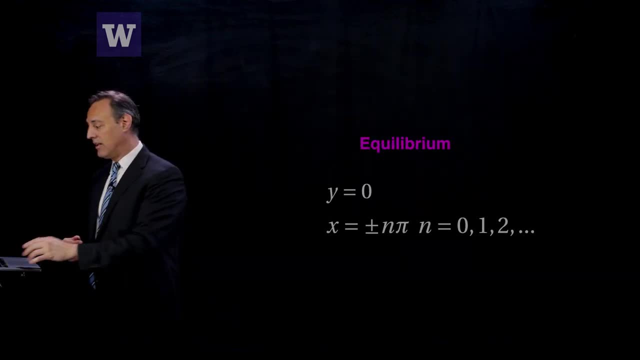 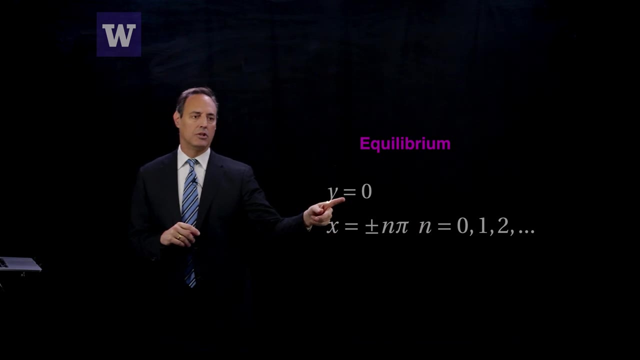 So I have actually an infinite number of fixed point equilibrium solutions, And what do these correspond to, these n, pi and the 0?? Well, the 0 corresponds to the fact that remember that y was equal to theta dot. In other words, there is no angular velocity. 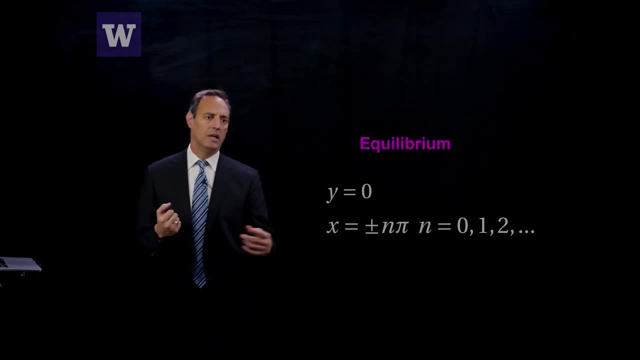 to this pendulum swinging around. And x equals n pi. 0 pi is when it's facing straight down, And 0 pi, 2 pi, 4 pi are the negatives of those, And pi, 3 pi, 5 pi. 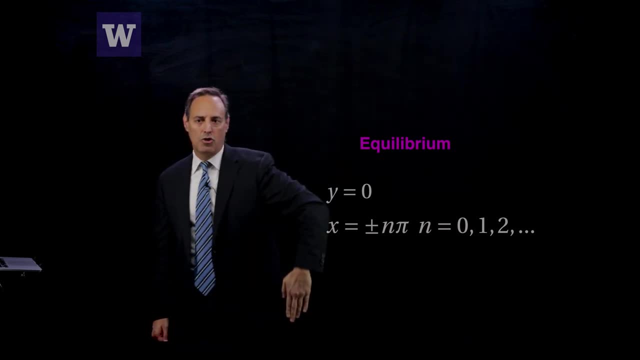 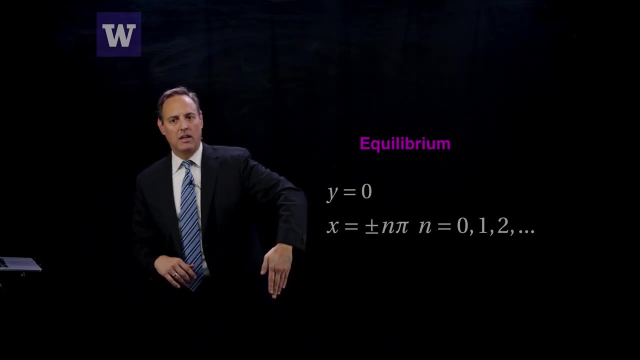 is when it's in the upright positions. These two positions are special. They're equilibrium points And right away you know that when it's in the down position, if you perturb it a little bit it's going to be stable right. 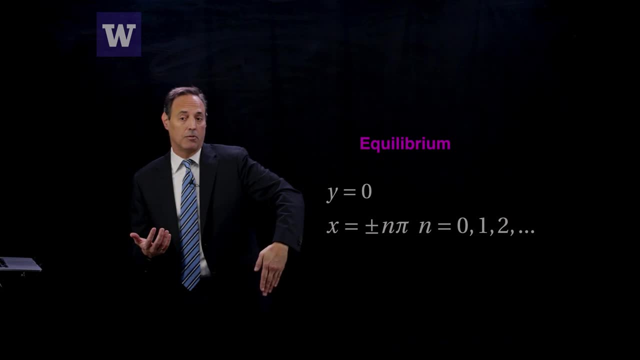 Because, in fact, if you perturb it a little bit, this pendulum will stay down here, will remain down here, While in the upright position the pendulum, if you perturb it a little bit, we know that it will fall over. 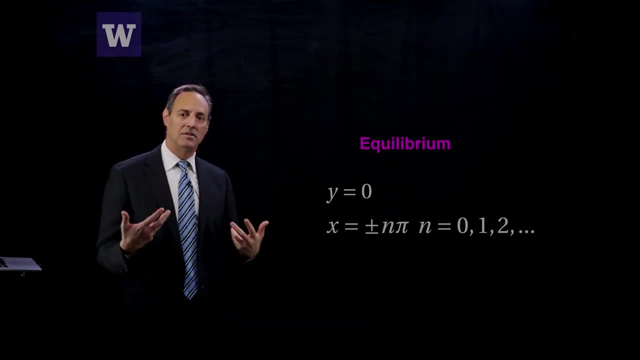 And so the upright position we already know should be unstable. The question is, how do we actually quantify that understanding of the pendulum? So we have to start looking at these equilibrium points as a start point, And the equilibrium points already tell us. 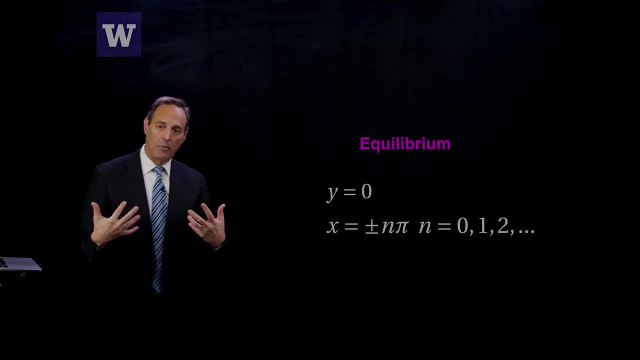 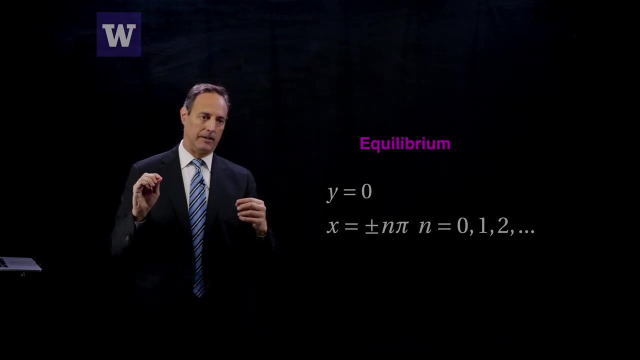 something very important. These are the very special points that we have to think about. in this nonlinear system where nothing is happening, where the dynamics is not moving, are these points Okay? So what we're going to do is we're going to start looking near these points. 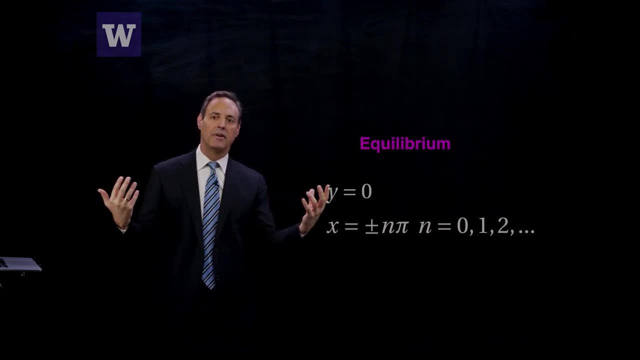 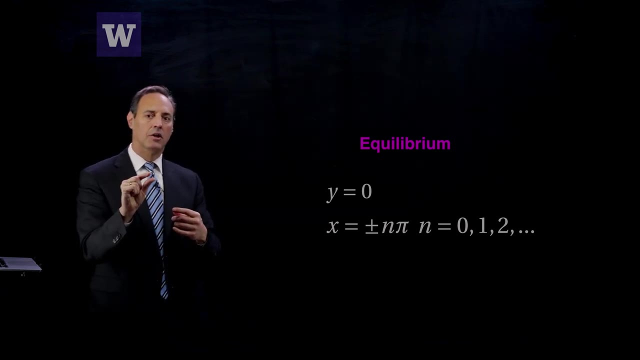 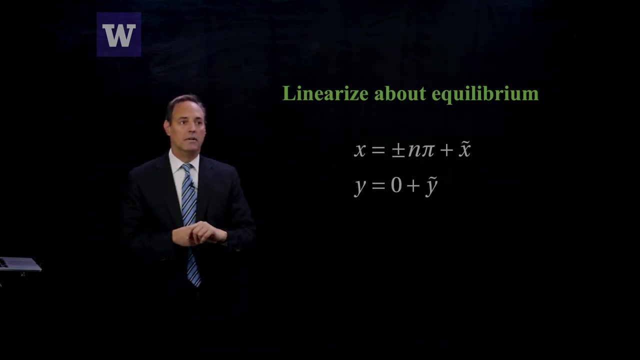 and taking this nonlinear system with an infinite number of fixed points, equilibrium points, and start looking at each one individually and look at a linear approximation near each. Remember the linear system only has a single fixed point. So here's how we do it. 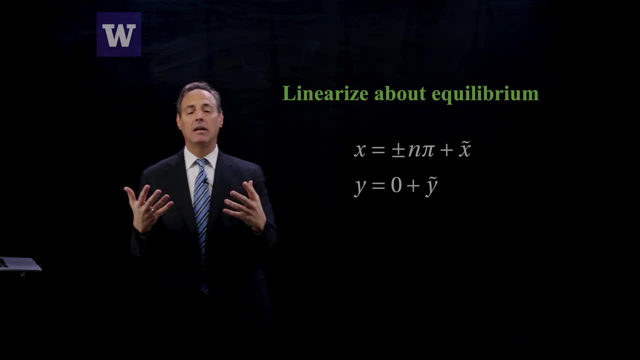 We linearize about the equilibrium points. In fact, this is exactly what you did perhaps in your beginning physics course. You took that sine x and you made it approximately x, And then we solve the linear pendulum. Okay, And many times. most people are familiar with the fact. 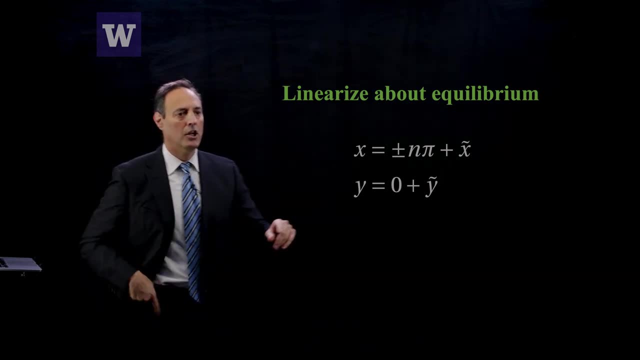 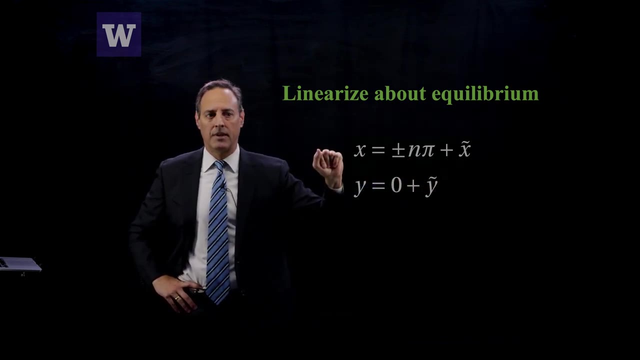 that you've already made a linear approximation to this problem. So here's how we're going to do it. here We're going to say x is equal to near one of these equilibrium points, plus x tilde, And y is going to be 0 plus y tilde. 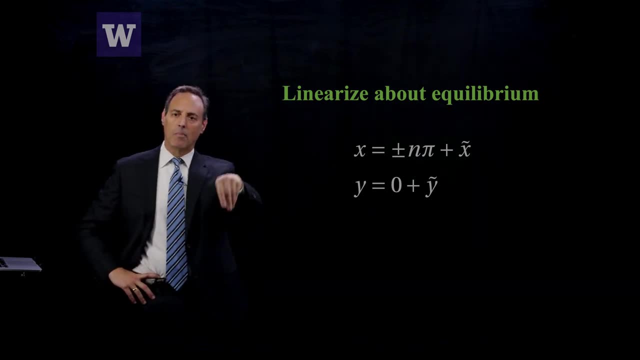 And the idea here is that x tilde and y tilde are both going to be very small, So they're going to be perturbations, So we're going to be very near the equilibrium points. Okay, And by being very near the equilibrium points, 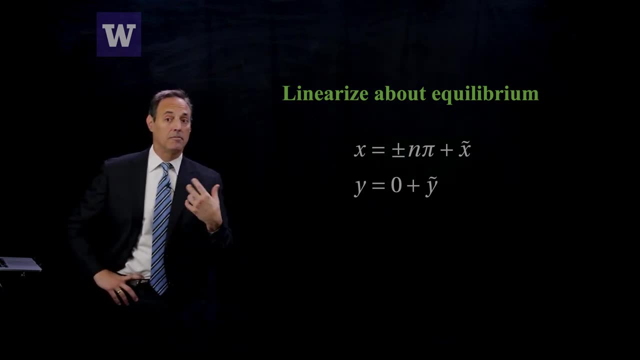 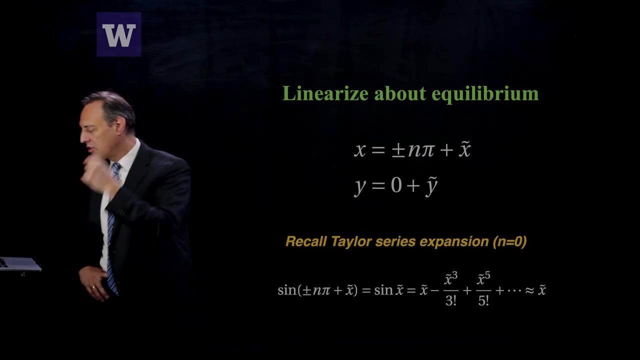 we're going to make use of asymptotics and perturbations to get us approximate solutions. So let's start off with the first piece of asymptotics you probably have already used, And this is exactly what we did, What we did previously with the pendulum. 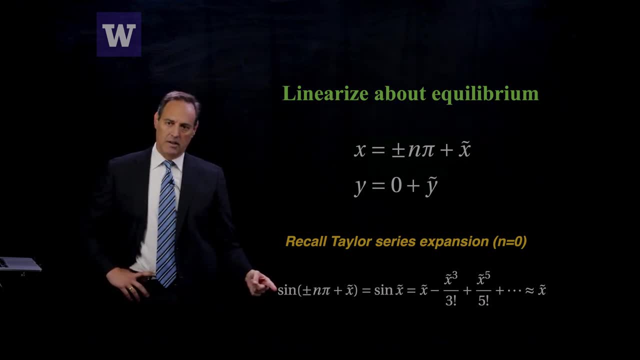 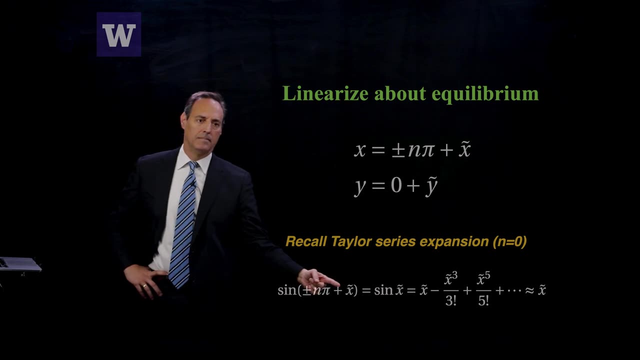 is if you say, if I'm going to expand here's this sine and I'm expanding this x around this equilibrium point, so it's plus or minus m pi plus x tilde Here it is. Well, if I do this around, n equals 0,. 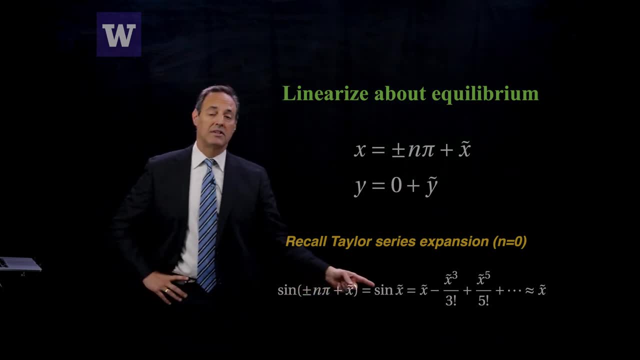 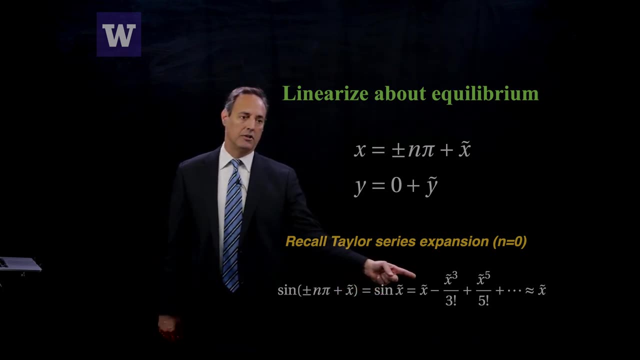 so I'll just throw n equals 0 down here. so then I have sine of x tilde and then I can just Taylor expand this. So I'm just going to do a standard Taylor expansion of the sine function and there it is. 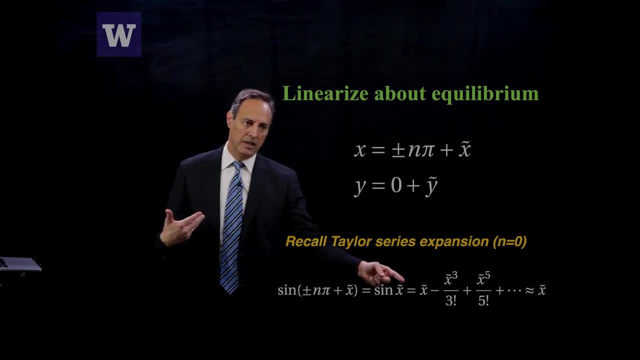 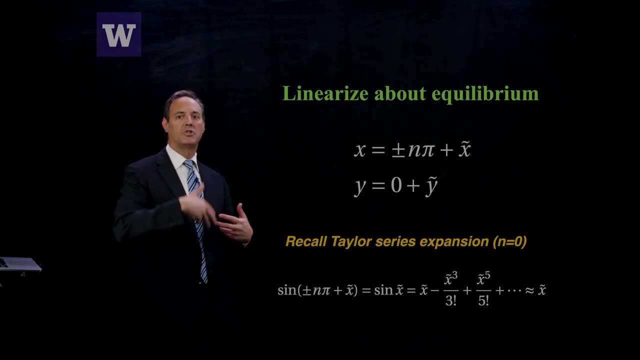 But notice what happens when I do a standard expansion: Sine x tilde is equal to x tilde minus x tilde cubed. Now suppose that x tilde is small, like 10 to the minus 2. Then the first term is 10 to the minus 2.. 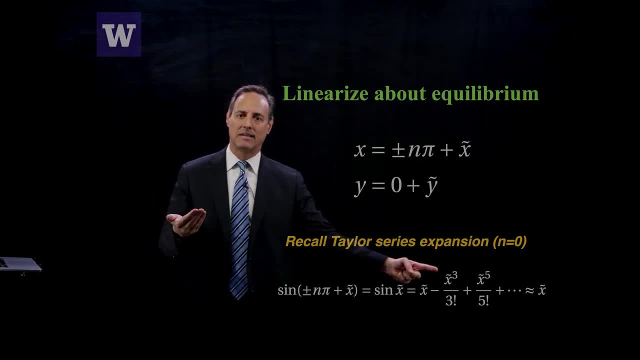 x tilde cubed is like 10 to the minus 6.. And this x tilde to the 5 is like x to the minus 10.. So you can see these are much smaller than the x tilde. So often what we do is then we say: 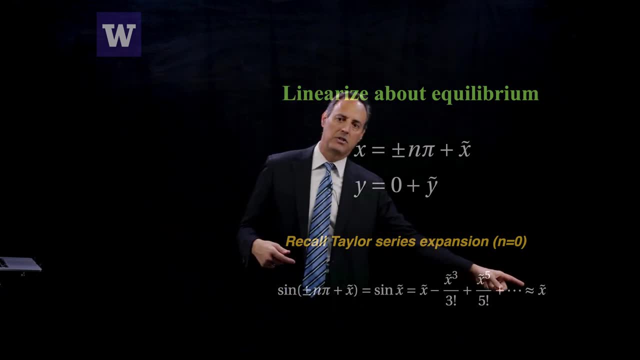 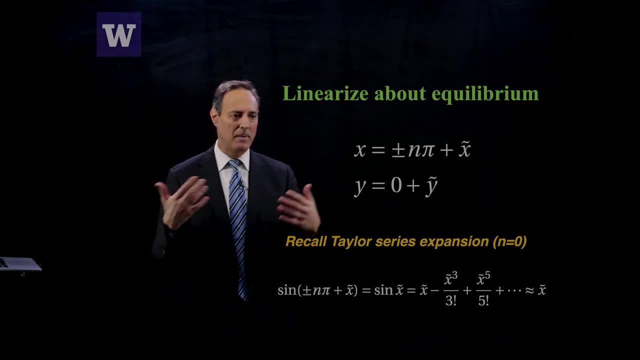 well then, I can approximate this whole thing just with x tilde, And this is exactly what we did when we first considered the pendulum in a physics course, is we said sine x tilde is about x tilde, and then we had a linear pendulum. 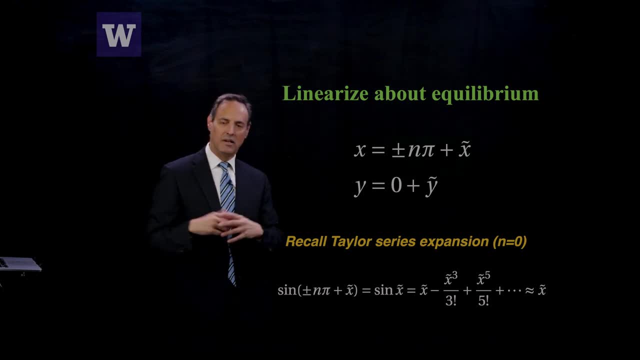 and this is why people think they can solve the pendulum. Well, it's an easy problem When you have the nonlinearity in there. it's not so easy, okay, But that's the whole basis of approximation that we want to be using here. 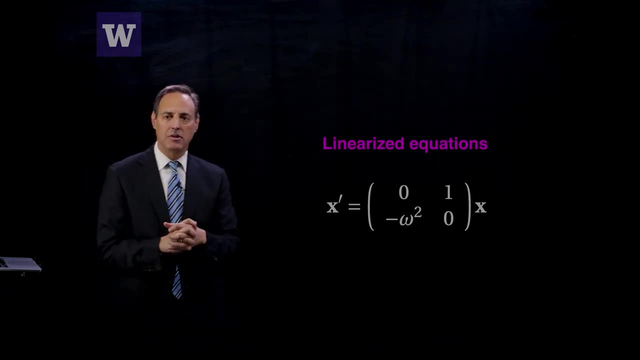 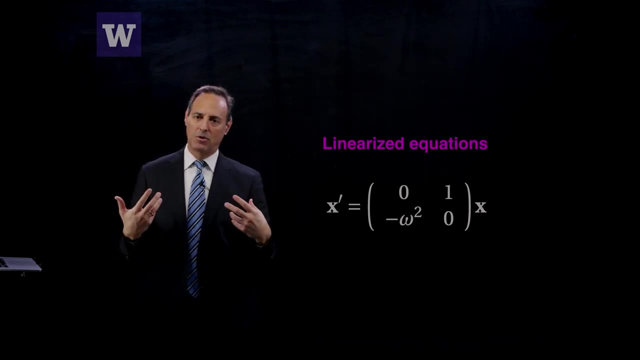 So if we actually take that approximation and put that back in, so sine x tilde is equal to approximately x tilde, then that 2 by 2 nonlinear system of equations becomes a linear system of equations. and here it is where x, here this is the bold x. 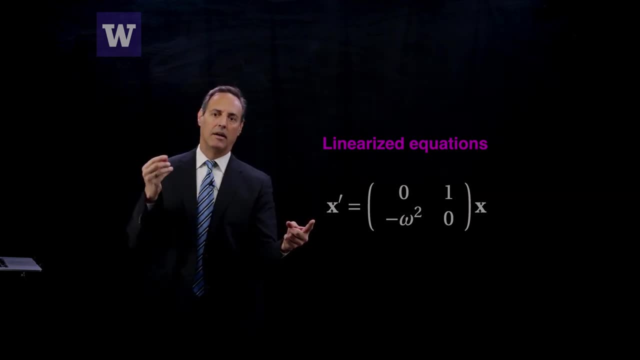 which is the two components, little x and y, which are the theta and theta dot. And so you get this 2 by 2 system of equations, and we've already talked about this as well. all I have to do is find the eigenvalues. 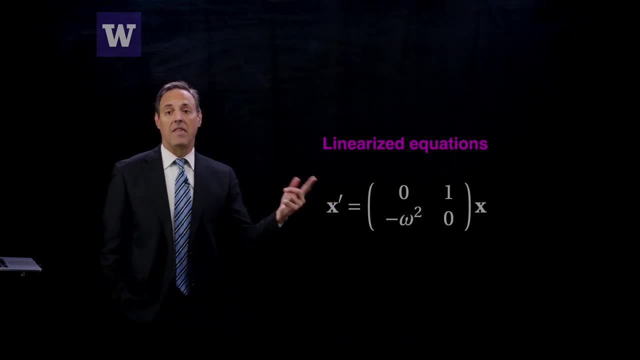 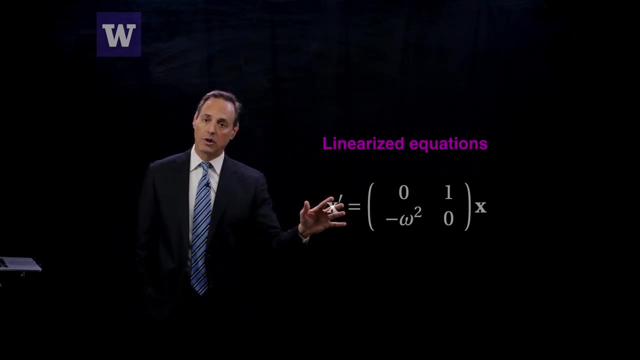 and eigenvectors of this. and then I have, and it's going to fit into one of the five forms that we talked about. So this is near the origin. So remember, we did expansion with the pendulum in the down position. 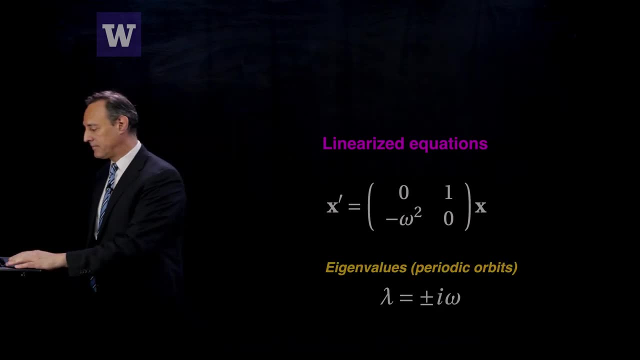 Here is our linear system approximation. And if you do your eigenvalues, compute your eigenvalues, what you find is the eigenvalues give you a center. In other words, the eigenvalues are purely imaginary. So if you now remember, we did this. 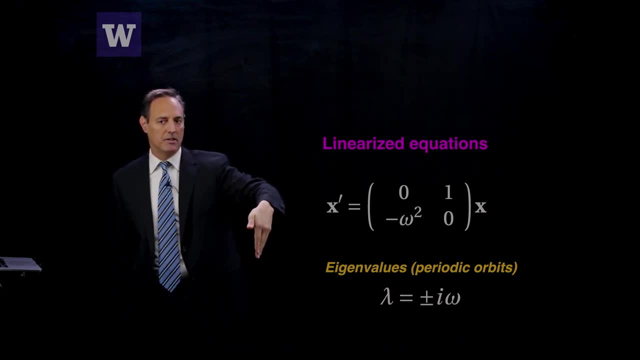 this is the approximation we did. We're near the bottom of the pendulum swing. There is no frictional forces, It's just no damping. So if you started oscillating, what this tells you is that the eigenvalues tell you that they are purely imaginary. 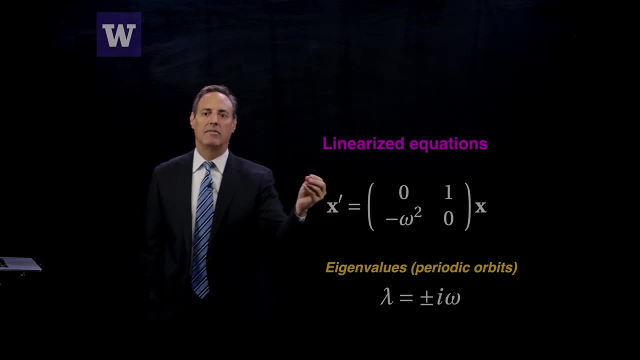 which means, in other words, the solution is periodic, forever, So it never will stop swinging, which, of course, once you have a little damping you'll go to zero, But initially at least, in this limit with no damping, if you start swinging this thing, 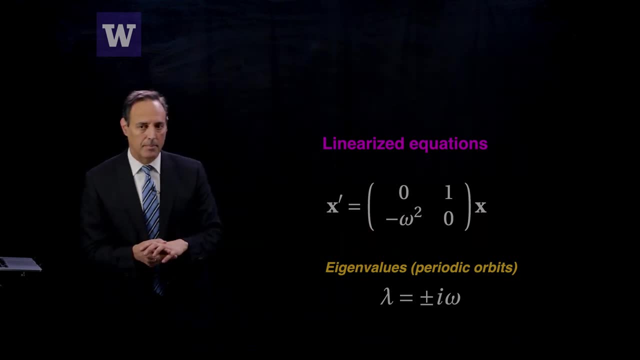 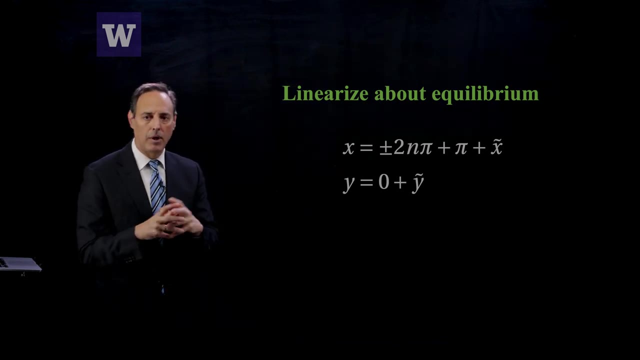 it will swing with a frequency omega, and it will not stop. So we can compute. So that's, and that's more broadly, how we would consider the system is like near that down pendulum, By the way, the down pendulum. 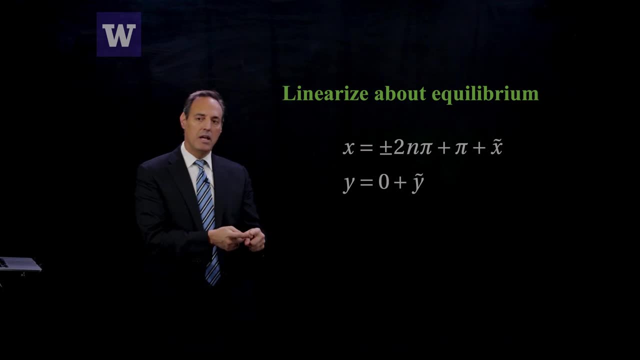 and also two pi multiples of it are the same thing. So two pi multiples. it's back in the down position and those eigenvalues are purely imaginary, always in that position. We can also look at it when it's in the up position. 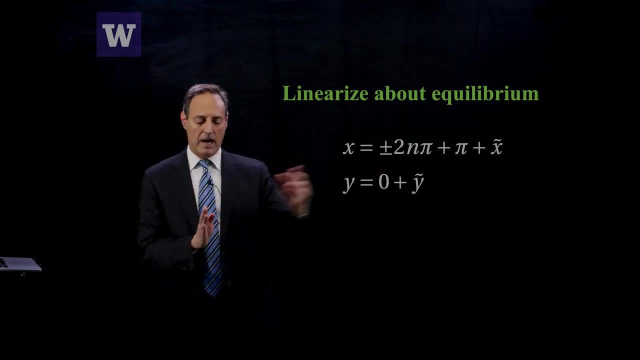 So now we're going to linearize about the equilibrium plus or minus two pi. In other words, I'm at the bottom of the swing, two pi plus pi. So I'm going to put myself right at the top. That's what that plus pi does. 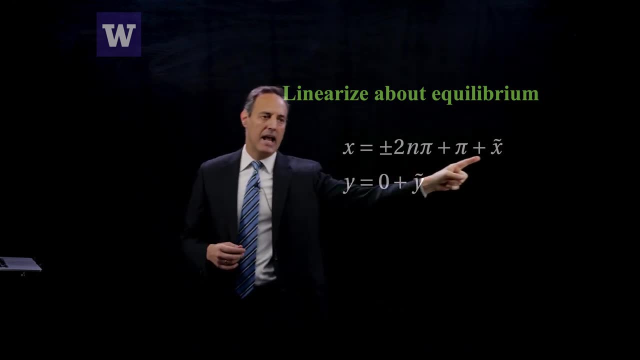 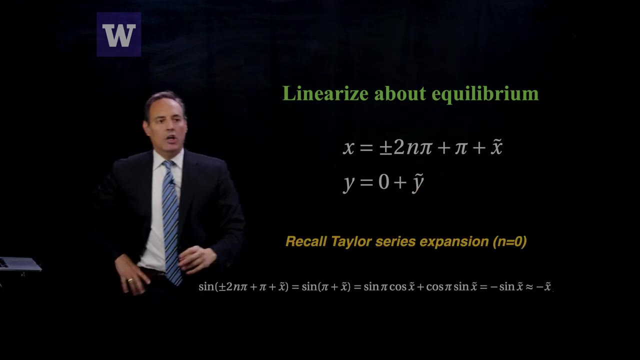 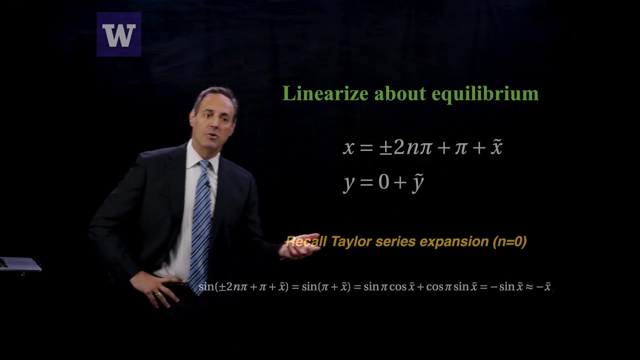 So now I'm going to take that value and add a little perturbation to it, And then y is still perturbed around zero. So recall from the Taylor expansion, it was around zero. We were able to Taylor expand, and now we're going to do it again. 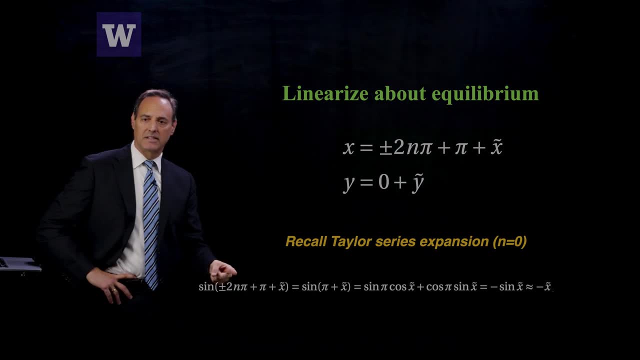 but we're going to Taylor, expand this or, look at, do some a little bit of fancy. you know some of our trig rules. We're going to now expand this thing. So here's your plus or minus n two pi. 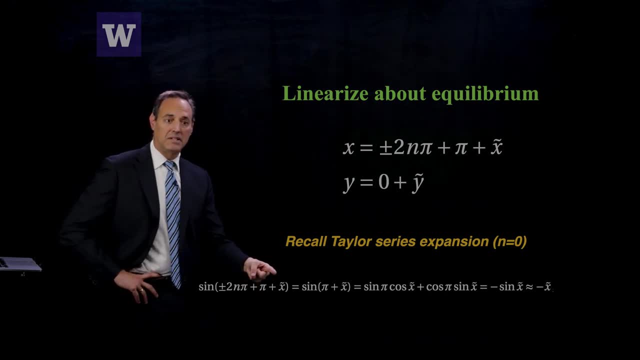 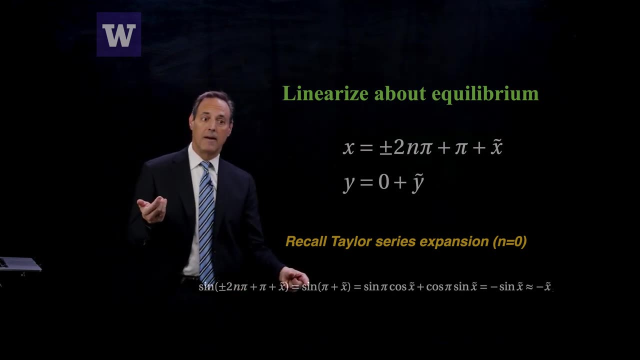 plus pi and x tilde, But you can basically this: two n pi does not matter, In fact, it's just two pi shift, which tells you that this is equal to sine pi plus x tilde, which now, if you use this trig relationship, 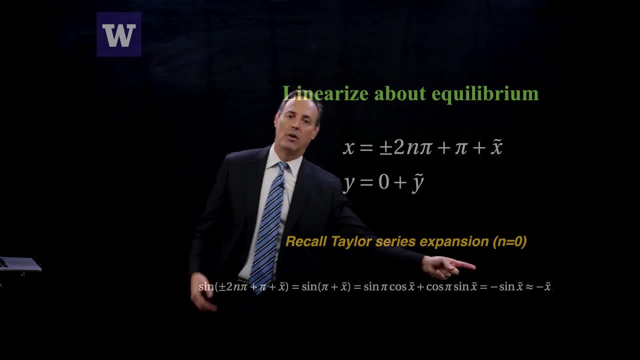 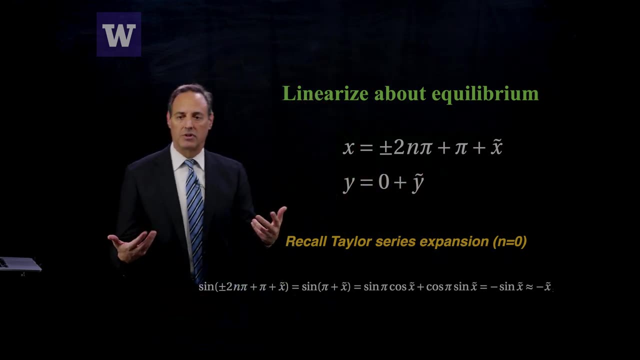 of sine cosine plus cosine sine, you find yourself in a situation which this is equal to now negative sine x tilde, which is equal to negative x tilde, when you do your Taylor approximation- So remember we had at the bottom sine x tilde- was equal to x tilde. 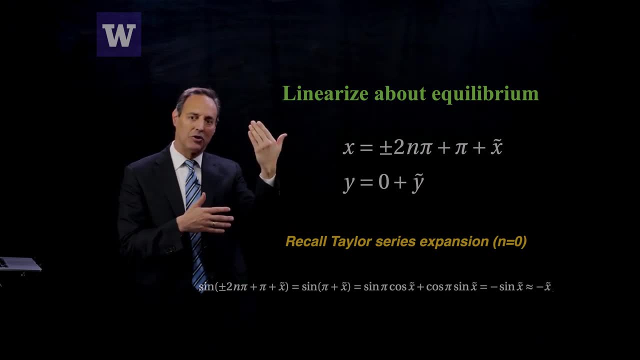 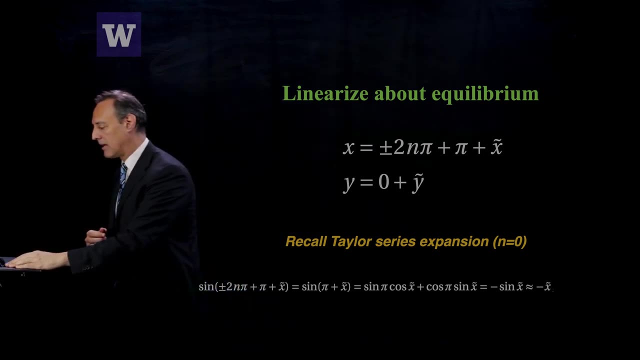 At the top, this sine of x tilde is equal to minus x tilde, So it's a sine switch, And the sine switch is going to make all the difference in the behaviors. So now your linearized system is given by this. 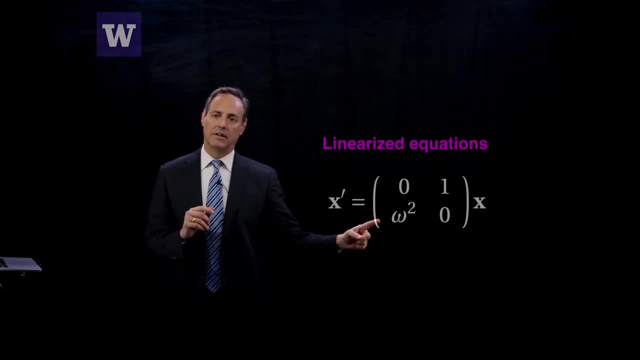 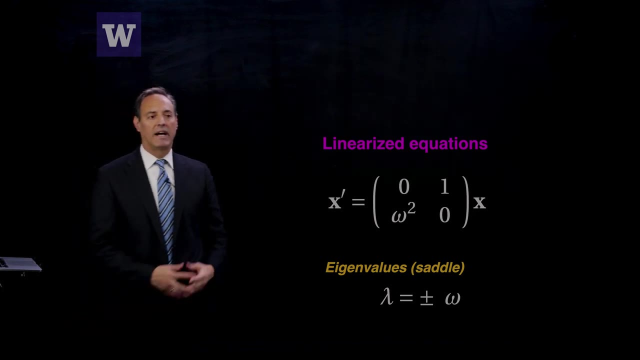 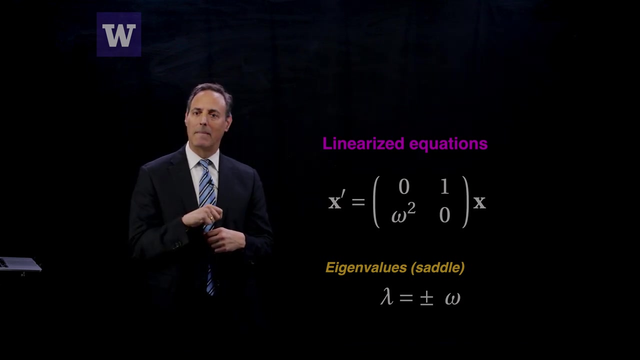 And the only difference from before is that before we had a minus sign here and now we don't. Now you can compute your eigenvalues And now the eigenvalues are purely real and they're opposite sign: One's omega, one's minus omega. 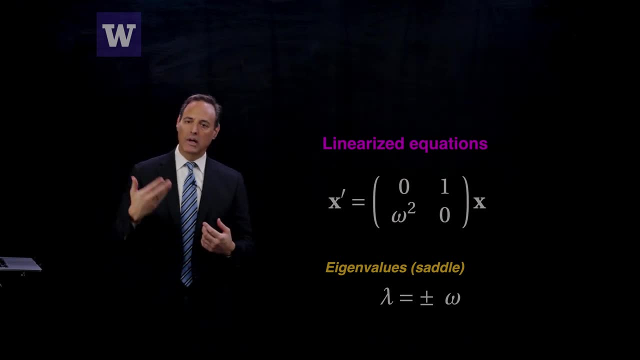 Here they are. So this is a saddle. There's one unstable direction and one stable direction. So that's going to tell us something very interesting, right? So when you're at the top of this pendulum, or when the pendulum's in the upright position, 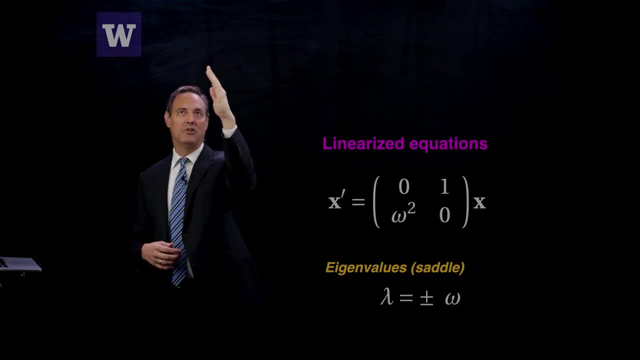 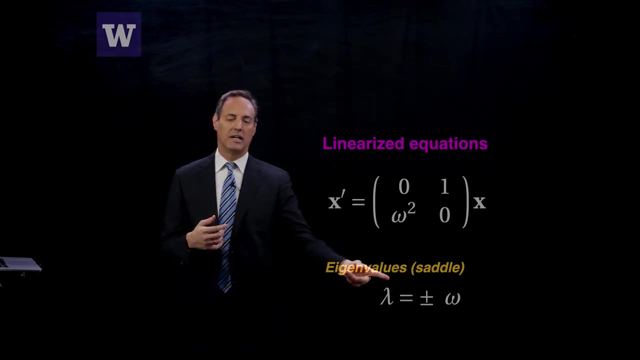 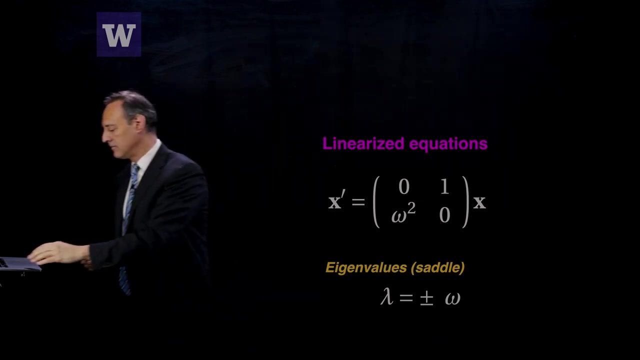 you come up to it, That's the stable direction, But then you fall away on either side and that's the unstable direction. Okay, So this is exactly what this is telling you, So you can get drawn into this fixed point, but then you eventually go away from it. 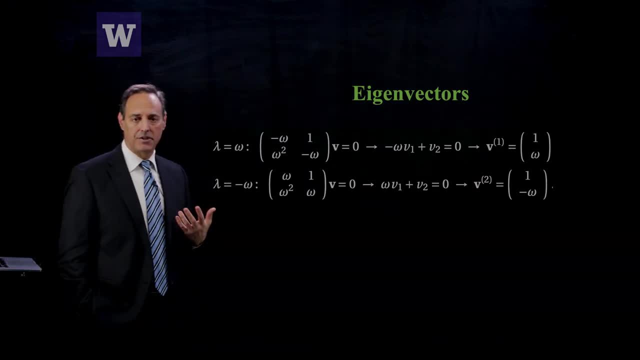 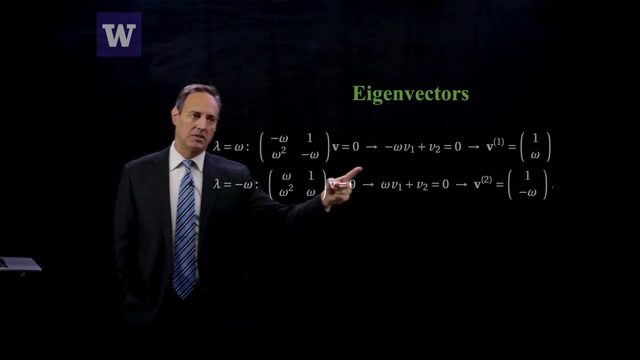 And here are the eigenvectors. And the eigenvectors for this are actually pretty nice, easy to calculate. Calculate the eigenvector for the omega case. So you put that back into a minus lambda ix. Put that in What your eigenvalue is. work this thing out. 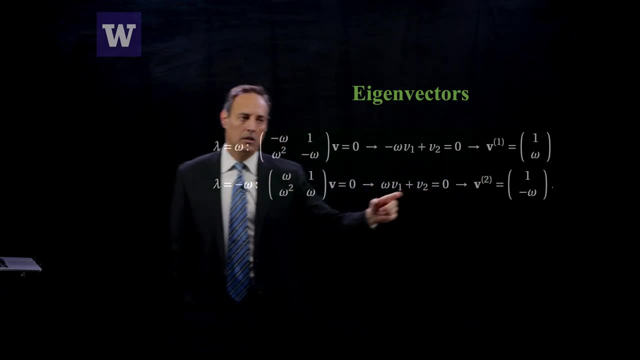 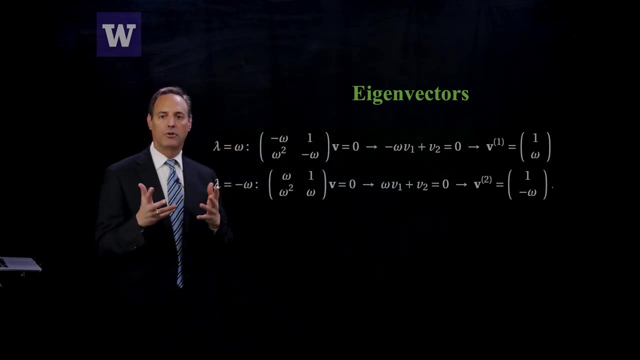 One of the eigenvectors is in direction one over omega. The other eigenvector is in the direction one minus omega. Okay, So you have your two eigenvectors. You can compute their directions for the stable and unstable directions around each of the fixed points. 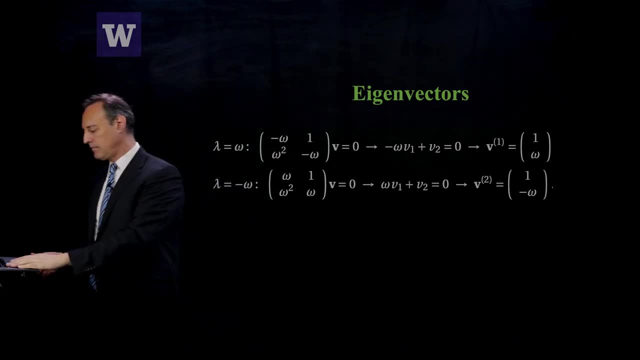 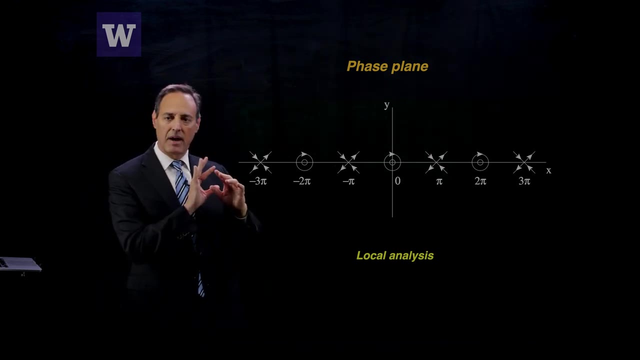 in the upright position of the pendulum. So here's what it kind of looks like. Remember, all of this was based upon perturbations. So here's, Remember I have an infinite number of equilibrium points And notice that what I've drawn here 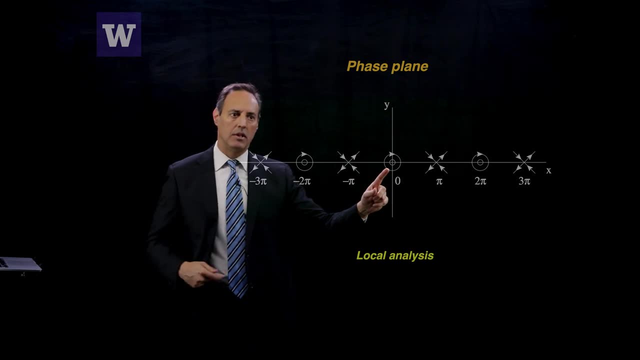 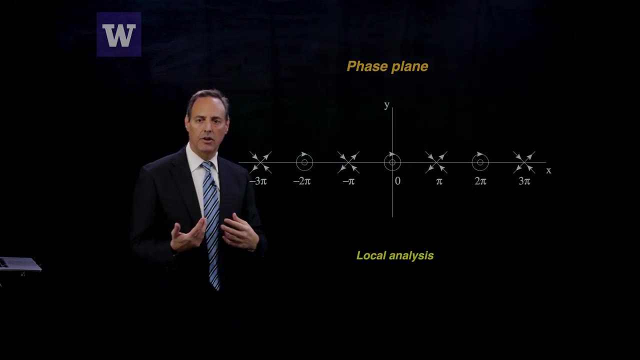 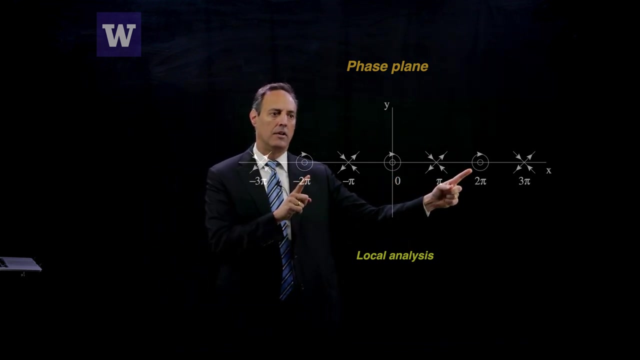 is that at zero, in other words the equilibrium point at zero, or multiples of two pi of it. what I found was that the behavior had purely imaginary eigenvalues. So what you see here is these things are centers There. they are just rotating around. 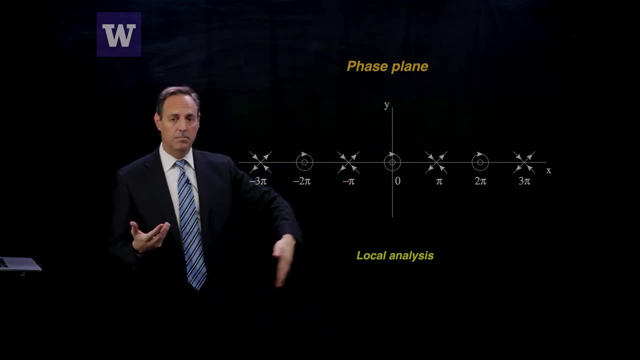 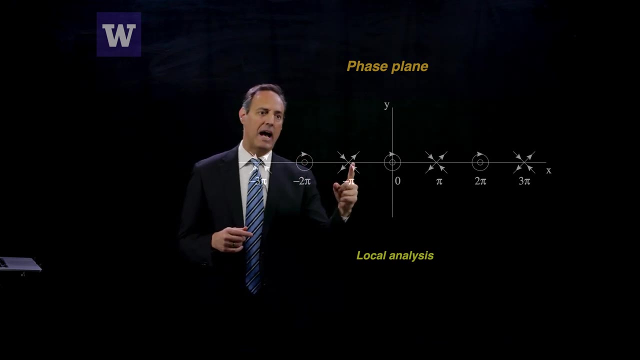 which is exactly what you expect. In other words, it's in this position, There's no damping, It will just oscillate forever, Whereas in the upright position and two pi's of that, that's what these guys are here, here and here. 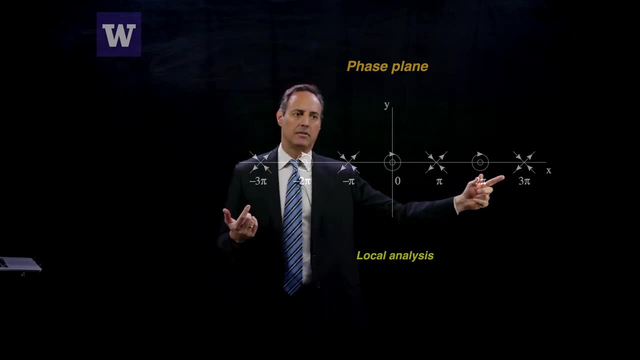 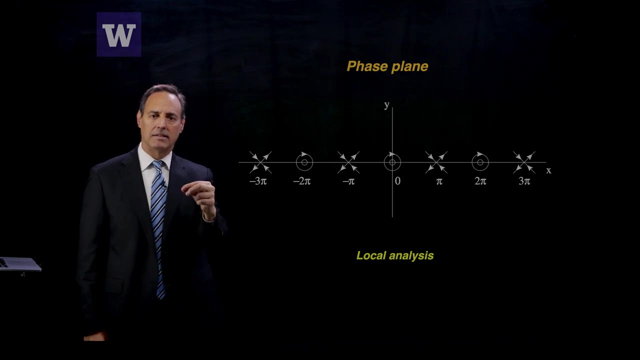 here, here They're saddles, So you have a direction in and a direction out. So all of this is a local analysis around each one of these points. The perturbation theory, remember, relies on this being an approximation. So what I've shown you here 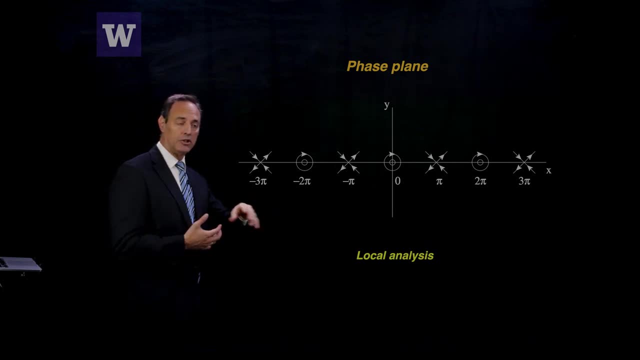 is the local analysis in summary. So this is what the behavior looks like for all these fixed points. Now, what we normally do, this analysis, because once we understand the fixed points and we understand their stability, we actually understand everything qualitatively. 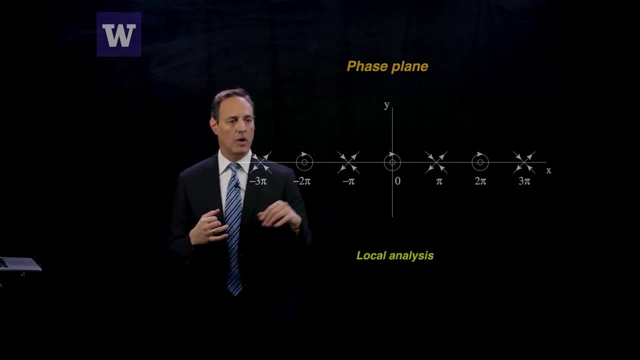 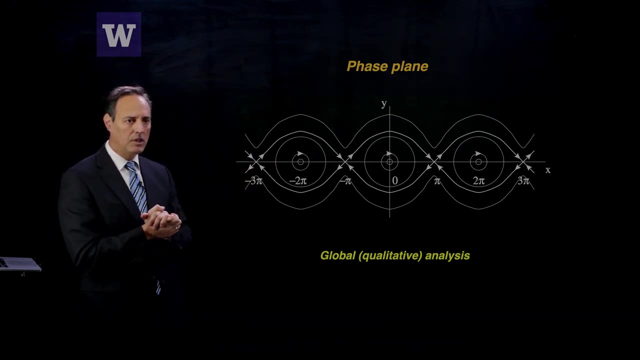 that can happen in this system In particular, if this is what happens on a local level, the only thing that can happen on a global level is something like this. So these fixed points like this and the only way for this to be self-consistent. 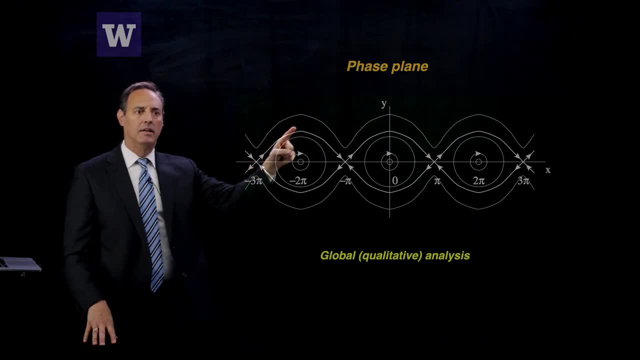 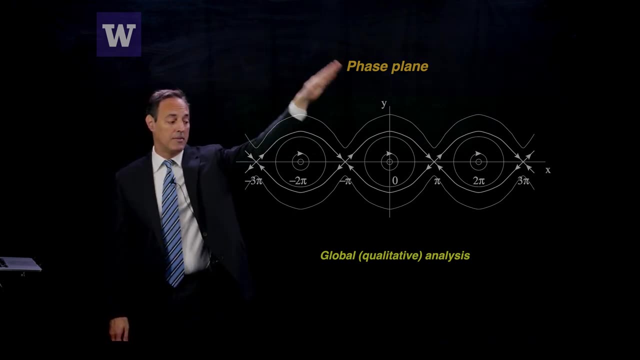 is the unstable direction of this guy ends up in the stable direction of that guy. So this is corresponding to when this goes from here, because the unstable direction comes around and ends up back up here at the top, And that's exactly what these 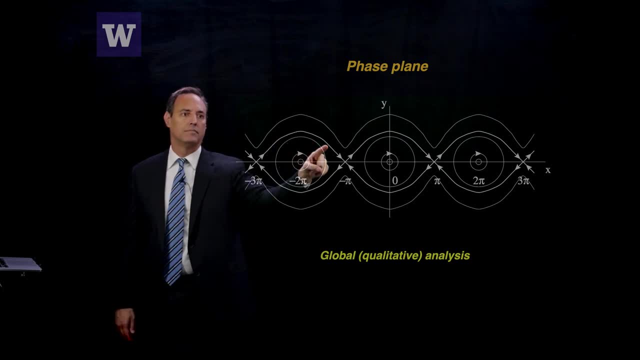 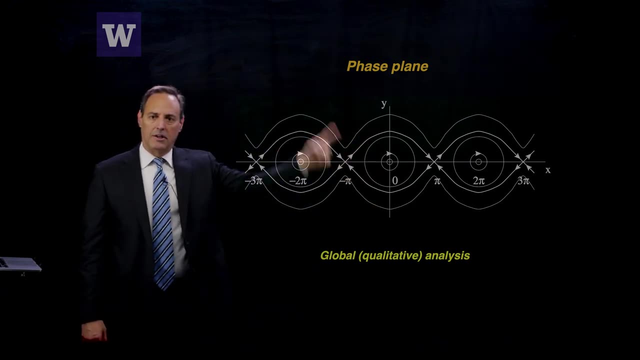 what are called heteroclinic orbits. tell us these trajectories. What these solutions are up here is, if you're rotating this thing and it just keeps going around and around and around, Remember it's not damped, So it just keeps going right by the fixed points. 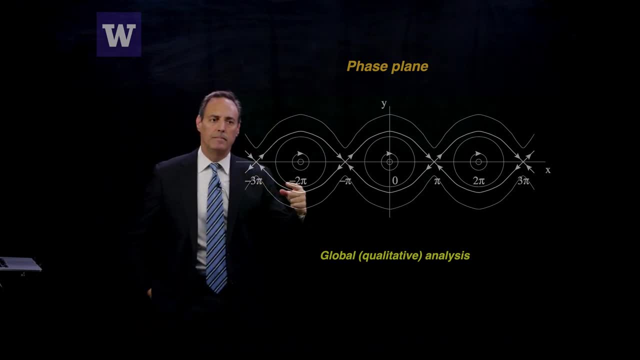 which are this direction and this direction. It just keeps rotating forever. And then if you're in here between negative pi and pi, then you're just simply oscillating inside this pendulum like this. So this is a question, a qualitative depiction of the dynamics. 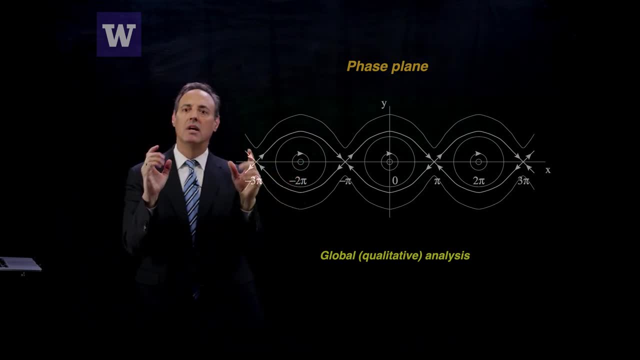 based upon your approximations of linear dynamics near each of the fixed points. Notice your perturbation analysis around each of the fixed points allows us to draw this qualitative picture and this is global. If you want, if you actually want quantitative analysis, then you could do. 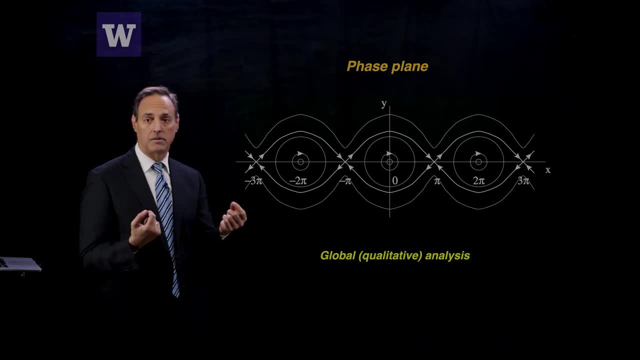 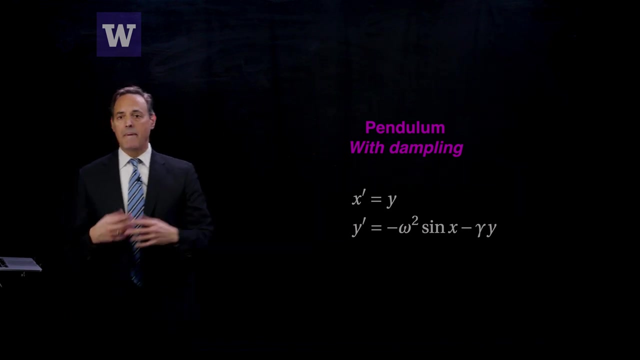 just go to recourse to numerical simulations, for instance. right, You can run these simulations And you can also write down solutions for the pendulum in terms of Jacobi elliptic functions. Okay, What about width damping? We'll finish this off. 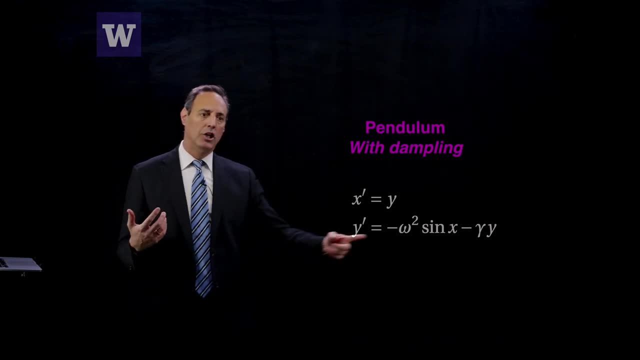 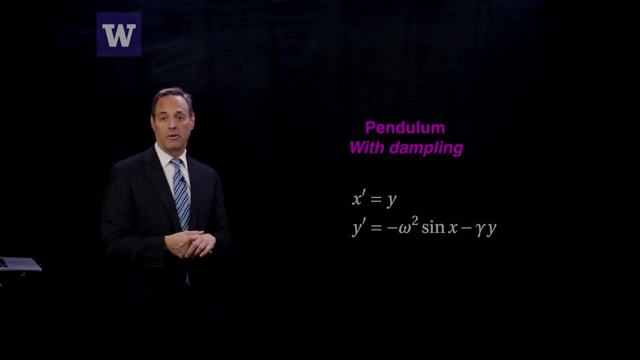 We'll bring the damping back in. So when you have damping, you bring this term back in, this minus gamma y, and you say: what are the fixed points now? Well, the fixed points are identical to what they were before, In other words, to make x prime equal to zero. 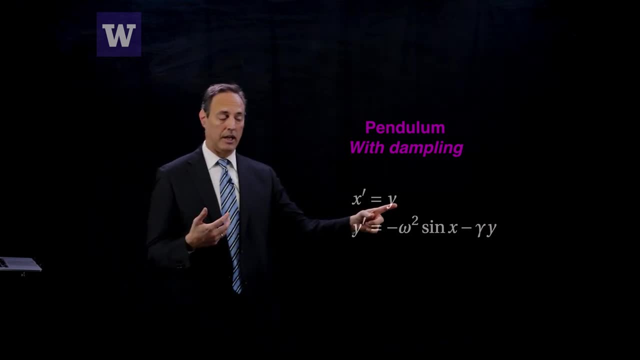 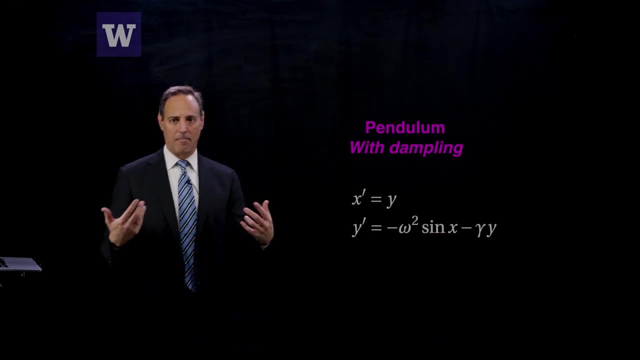 you have to have y equal to zero, which means this is y equal to zero here, y equal to zero here. To make y prime zero, then you have to make sine x equal to zero, which is plus or minus n, pi, Same thing as before. 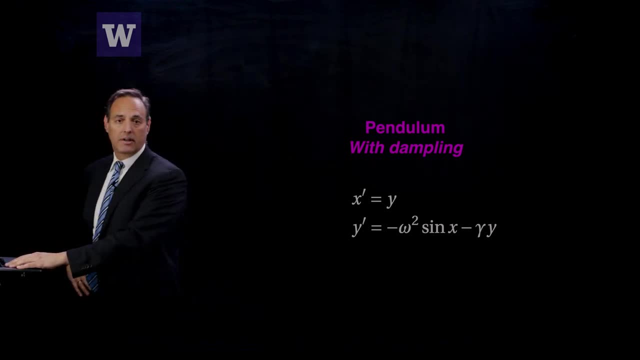 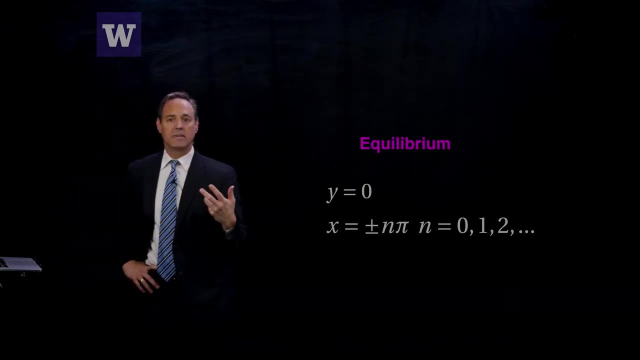 We have an infinite number of fixed points, and they're at the same locations as without damping, And so there they are. There's the equilibrium point. So I have everything the same, except for now, when you're going to compute your eigenvalues. 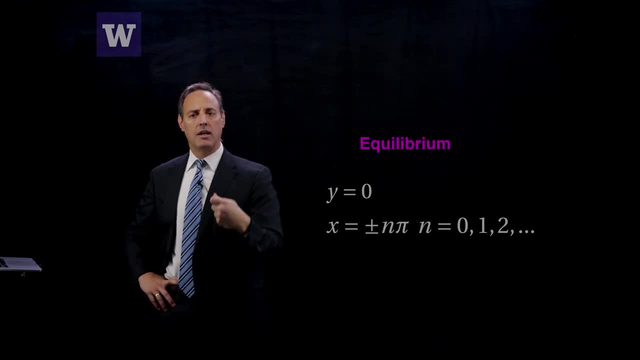 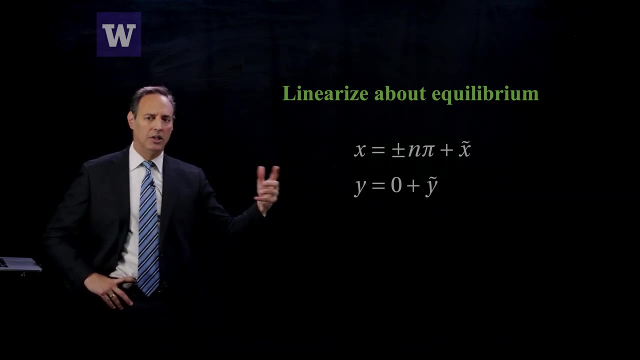 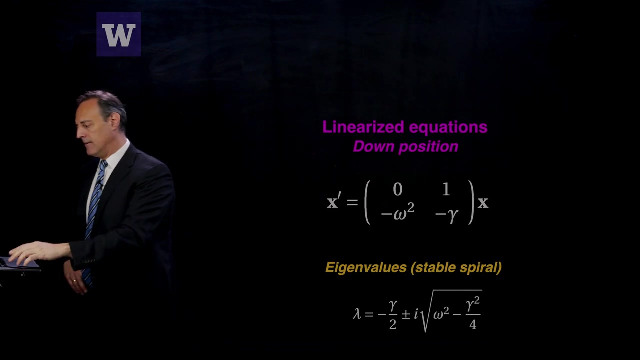 the presence of this damping term is going to change the eigenvalues. So here we go, If I linearize about the equilibrium, just like we did before. so a perturbation. so we're going to basically do a little local analysis around each of the different fixed points. 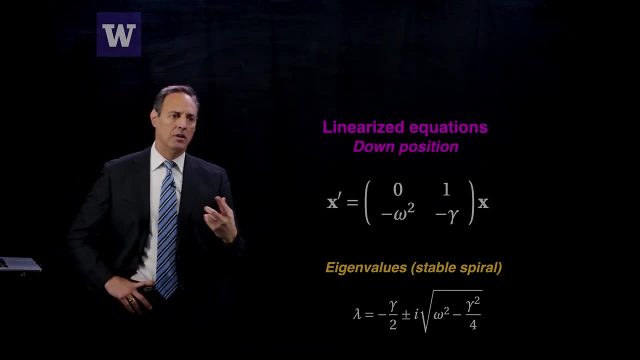 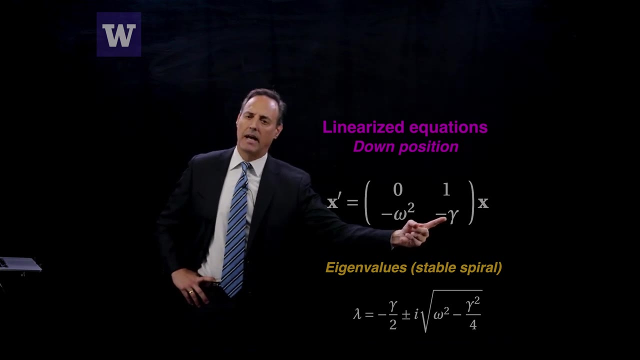 And if you linearize around the down position, here's what now the two-by-two system looks like. So now, the only difference here is- I've picked up this off-diagonal term minus gamma here, and when you compute the eigenvalues of this, 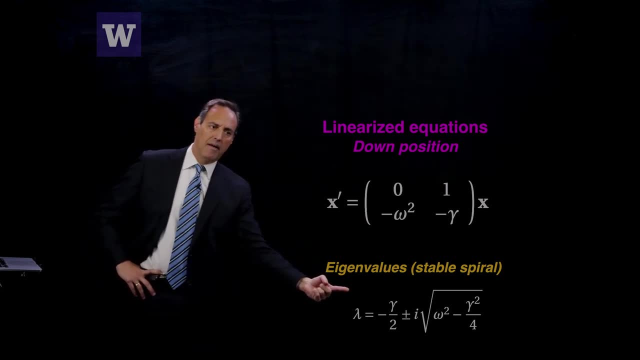 here they are. The eigenvalues have an imaginary component there, right over, on the right there, and this damping term minus gamma over two. So the real part is negative. so it's going to be damped and it's going to be oscillating. 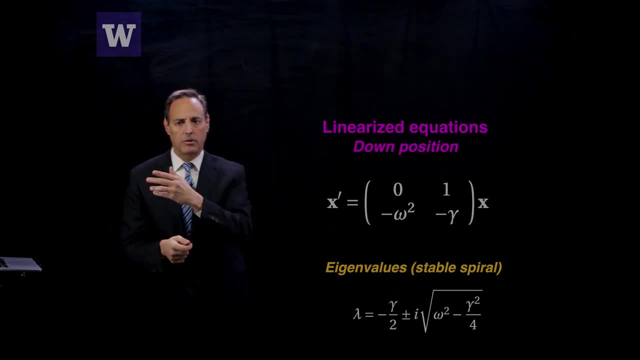 at that frequency, right there. So, in other words, it's exactly what you expect. If you start this pendulum off, it's going to slowly die down and end up at the fixed point, which is the down position. So this is the eigenvalues. 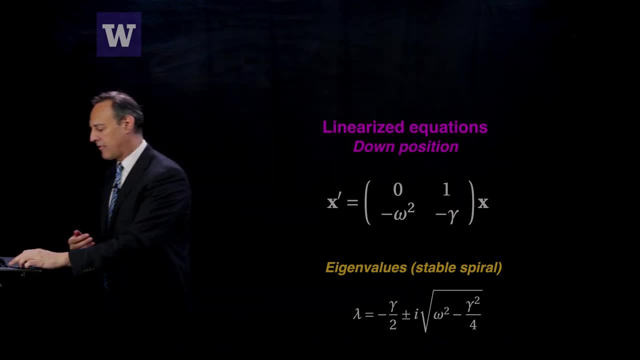 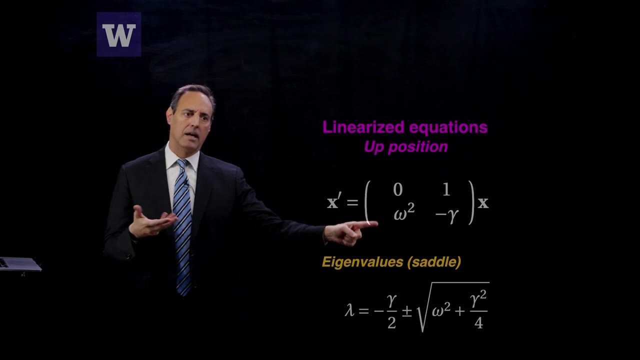 and this were all of the down positions, And if you do the same thing for the up positions, the only change here was that. now, remember this was a minus sign, now it's a plus sign. The eigenvalues are given by here. 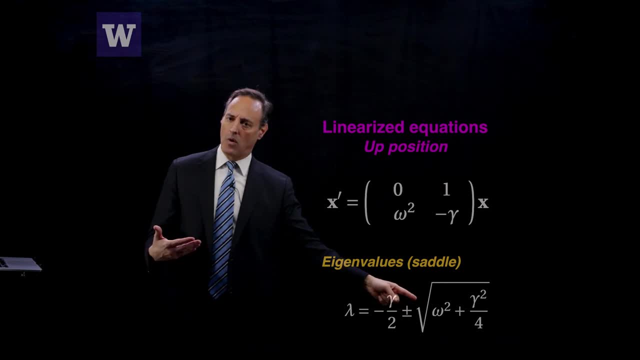 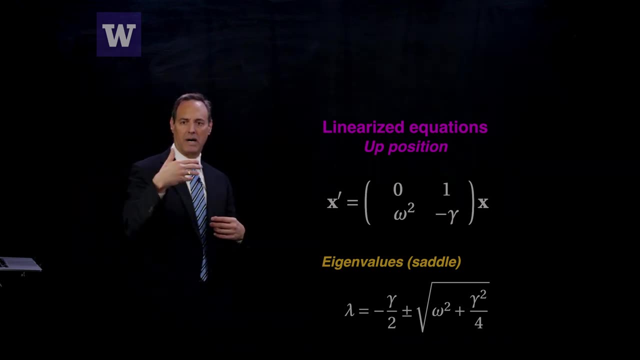 which now, this is square root of some positive quantity, and so there's no imaginary component and in fact you can find that one of the eigenvalues is positive, one of the eigenvalues is negative. That's pretty easy to see, right here, right? 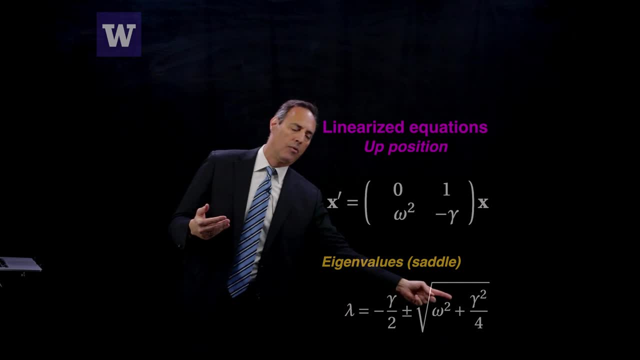 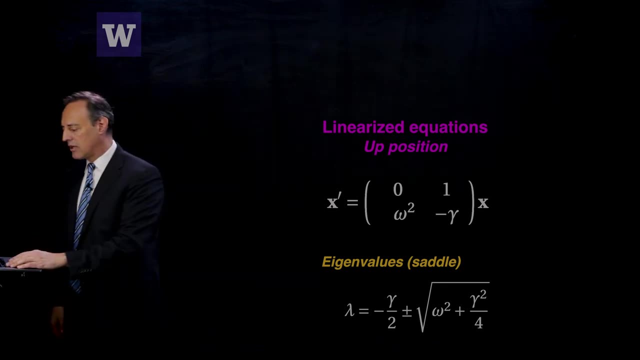 Because you're taking the square root of omega squared plus gamma squared over four. so this is bigger than this here and it's plus or minus. so you have a stable and unstable direction. That's your canonical saddle and your picture gets modified to this here. 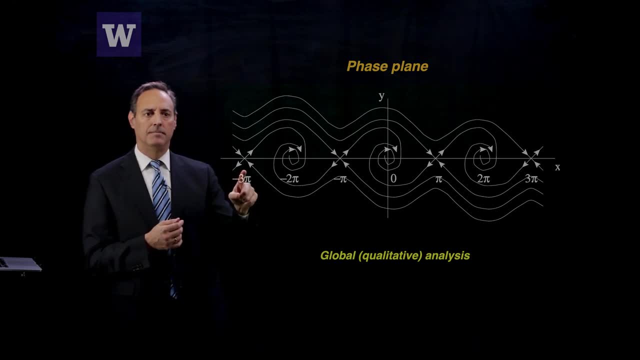 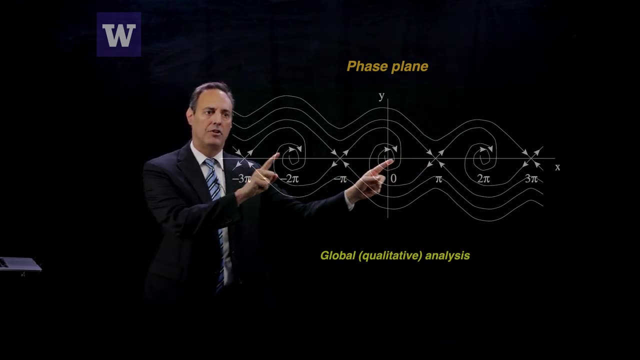 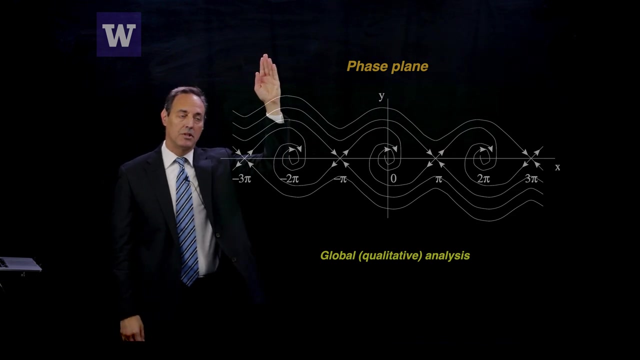 So now again, you have a saddle here and in fact here, and every two pi from it. this is the up position, and then you have here: these are your stable spirals. So in other words, if you start the pendulum from the upright position, 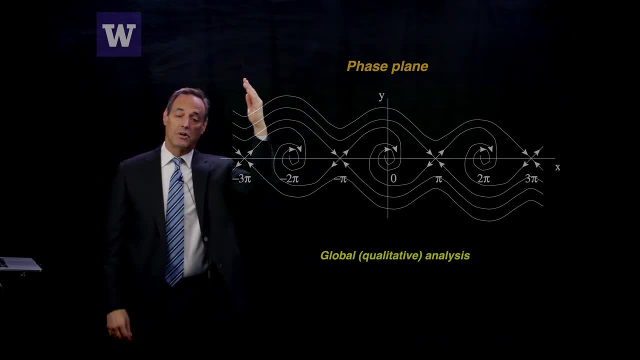 it will never get back up to the full upright position because you have damping. So instead you come down, you get some damping and now you just oscillate right into the fixed point. and that's exactly what these trajectories are representing. And if you really whip this thing around, 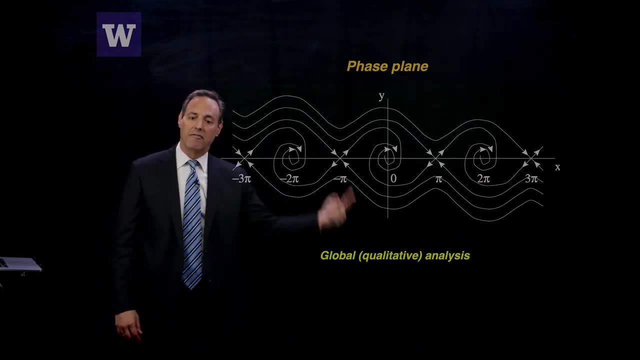 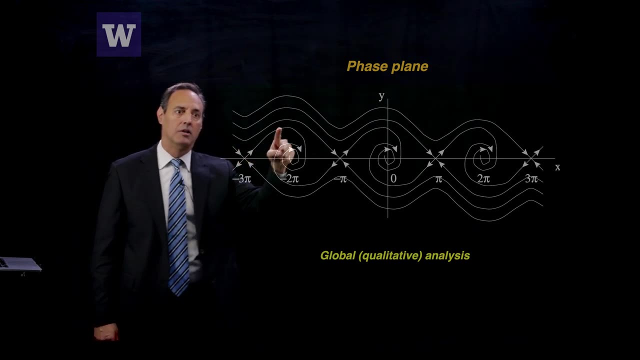 so it goes around several times and then eventually it stops and oscillates down to the bottom. that's what some of these trajectories up here represent. So in other words, here this one here comes down, comes down, oscillates twice around. 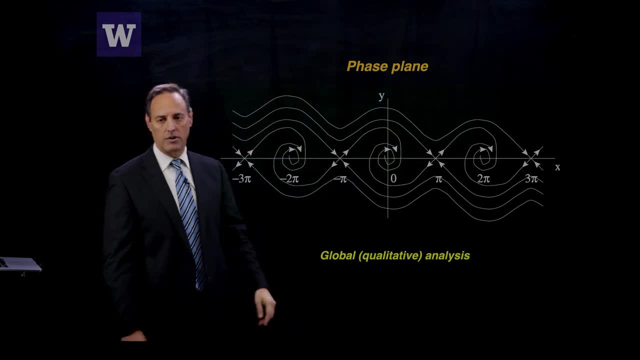 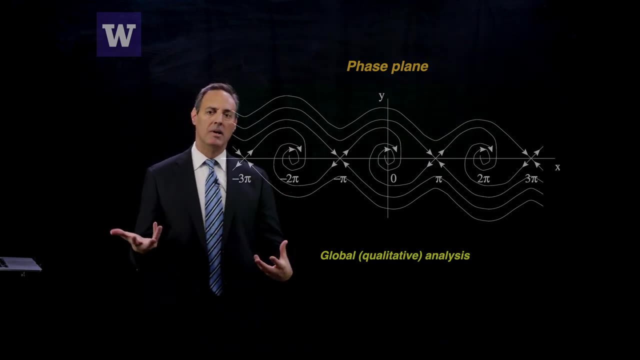 and then eventually it's going to get sucked in to one of these orbits. So this is our global understanding of the damped nonlinear pendulum, by doing local linear analysis and relying on approximations and perturbations to give us all the information we need. 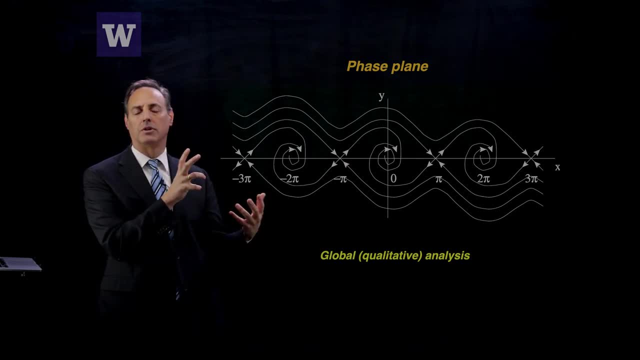 to construct this picture of what the solution looks like: The quantitative trajectories. like I said, you can just run this through simulation, but you already know everything that's going to happen qualitatively, And this is exactly what we're going after in many of the approximations. 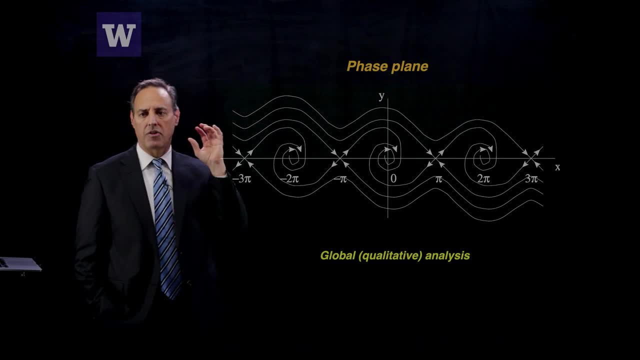 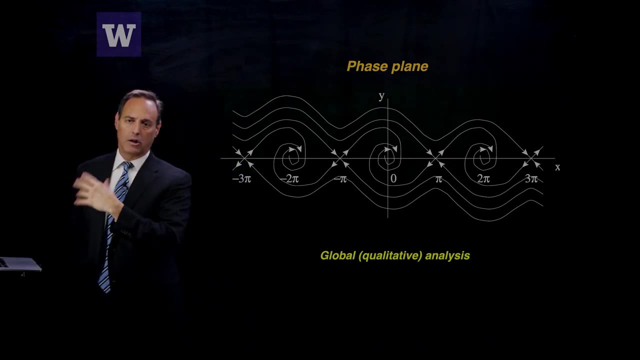 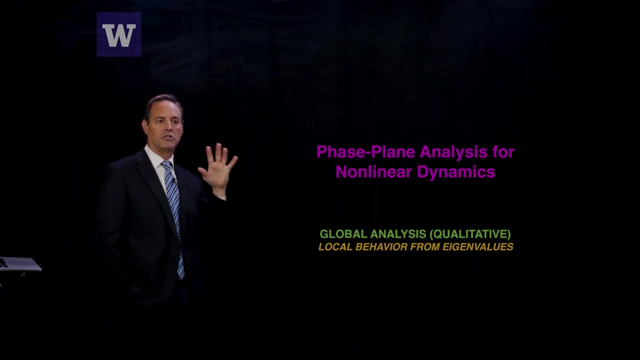 that we're trying to make for this course is we want to start thinking about how do I capitalize on all this local information to get me information on a global level so I can understand the problem very well. So here's the summary. The phase plane analysis was these nonlinear dynamics.